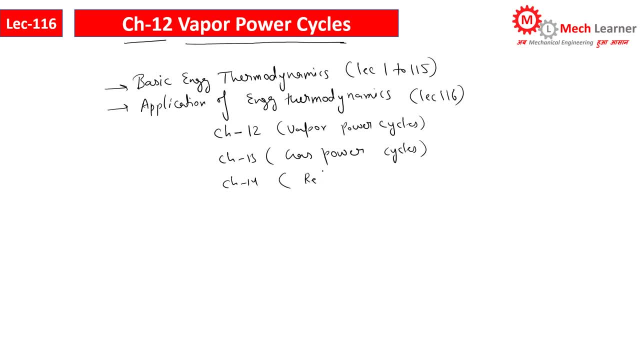 Chapter number 14, in which we will discuss about refrigeration cycle, Chapter number 15,, which name is Psychrometric. These two chapters are in RAC And this Vapor Power Cycle is in Power Plant Engineering, So we will discuss the same topic in Power Plant Engineering. 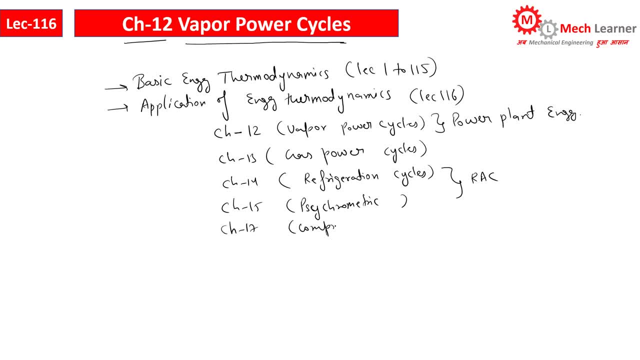 And last we will discuss chapter number 17, compressible fluid flow. So we have to discuss total 5 chapters. So in this video we will start chapter number 12, Vapor Power Cycle. So first of all we will discuss Thermodynamic Cycle. 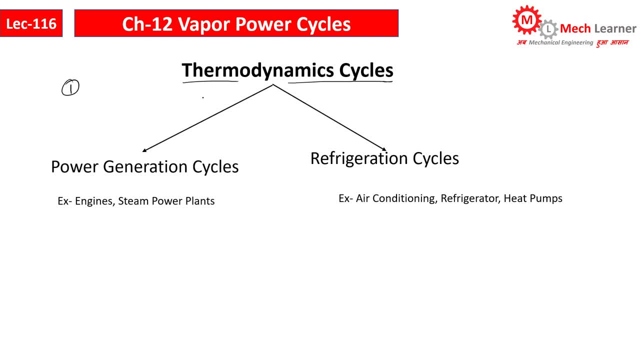 There are 3 categories of Thermodynamic Cycle. The first category is classified into two parts: Power Generation Cycles and Refrigeration Cycles. Examples of Power Generation Cycles are Engines, Steam Power Plants, Nuclear Power Plants, Jet Engines, Jet Propulsion Engines. 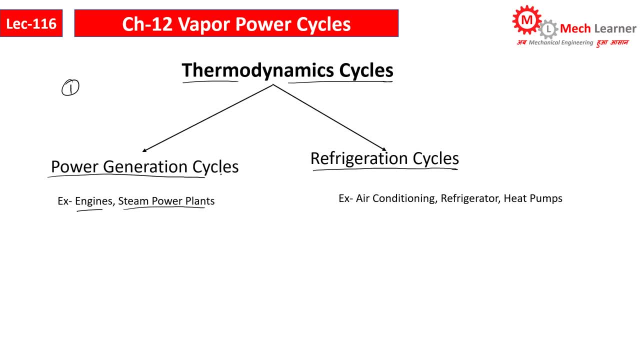 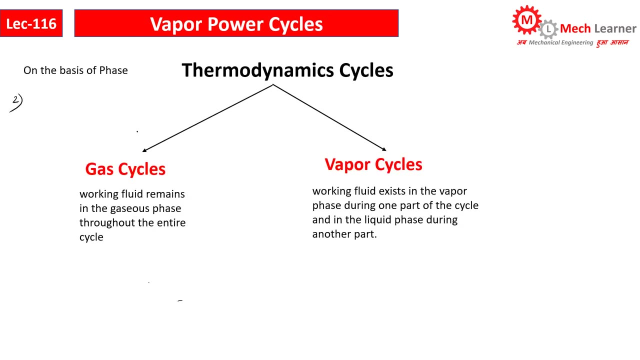 So all the engines with which we generate power are in the category of Power Generation Cycle. The second type of Thermodynamic Cycle is called Refrigeration Cycle. Examples of this are Air Conditioning, Refrigerator, Heat Pumps. Next we will look at the second classification of Thermodynamic Cycle, which we have divided into two parts. 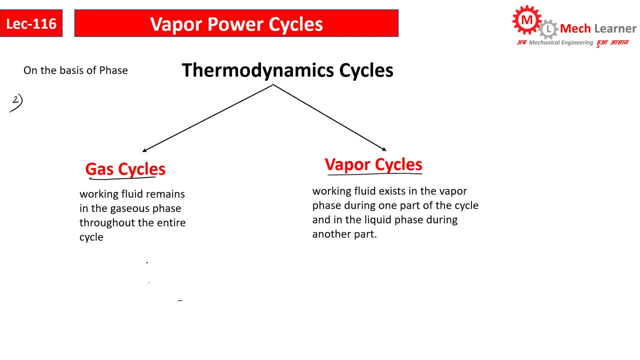 Gas Cycle and Vapor Cycle. What will happen? in the gas cycle, The phase of the working fluid in the cycle will be of gaseous nature. Phase 1 will be of single phase and its nature is of gaseous nature. In the vapor cycle, half of the working fluid will be of liquid nature and the other half of the cycle will be of vapor nature. 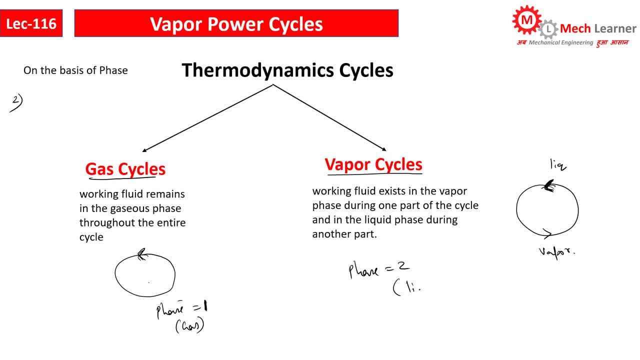 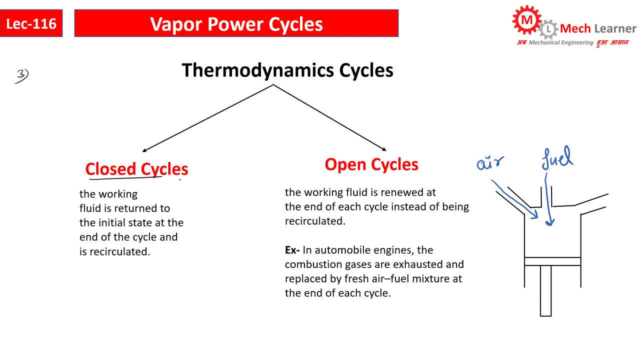 So here the total phase is 2. Which are Liquid and Vapor. Next we will look at the third category of Thermodynamic Cycle, which we have further divided into two categories: Close Cycle and Open Cycle. Close Cycle means the working fluid is returned to the initial state at the end of the cycle and is recirculated. 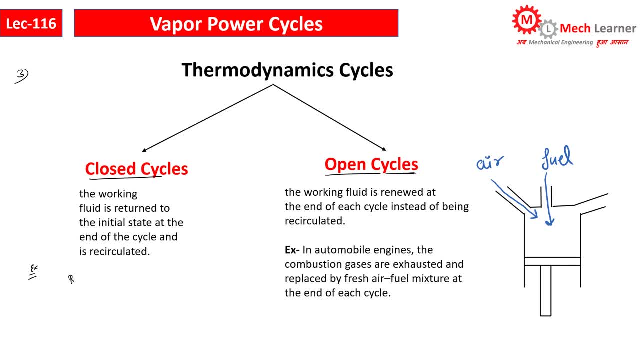 les see the two pinned factors, how they are inclined towards the initial state. Now here the method of which the scheme has started. For example, the team power plant, without using the boiler, working fluidice is pumped into the turbine. component00 wai is protested from the turbine into the condenser. 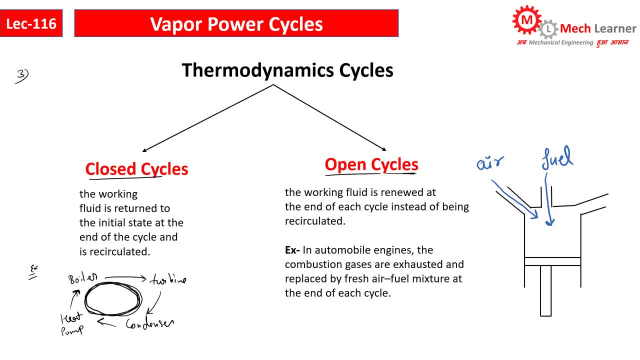 and donorます. Now, in open cycle, the working fluid is renewed at the end of each cycle instead of being re-circulated. In this cycle, one cycle is completed like this: In one cycle, the air-fuel mixture that is added to it after burning it is removed through the exhaust. 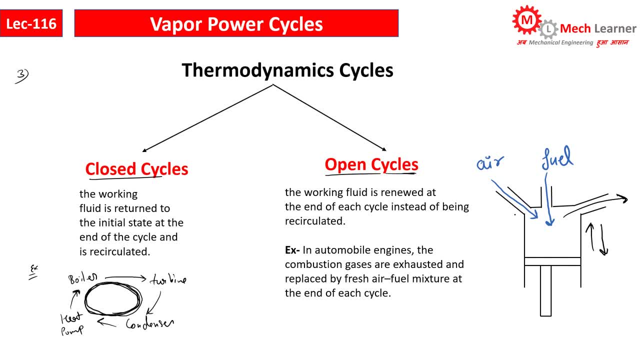 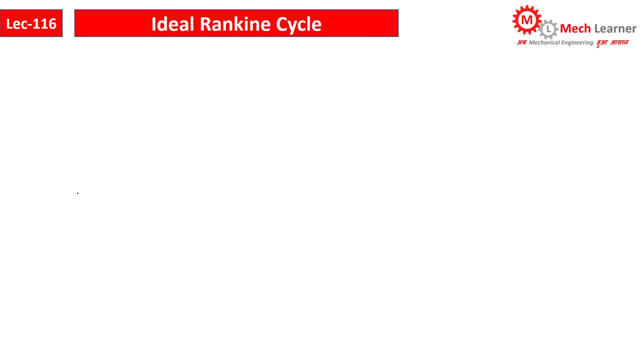 Now in the next cycle, the second air-fuel mixture will be added. So in every cycle the air-fuel mixture keeps changing. So this is an example of open cycle. Next we will understand the working principle of the steam power plant. 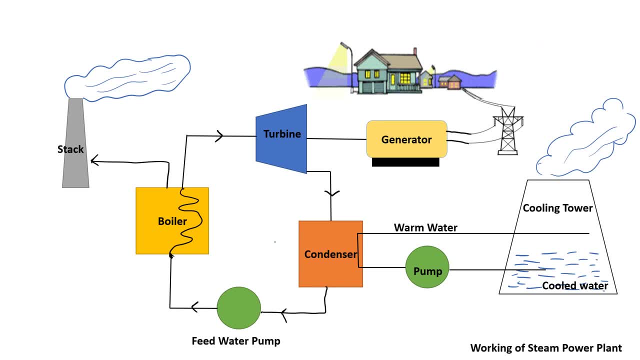 So in any steam power plant there are four main components: Turbine, condenser, feed water pump and boiler. The arrangement is similar: Turbine condenser, feed water pump, boiler. This is how the cycle is, And the cycle used in it is called the vapor power cycle. 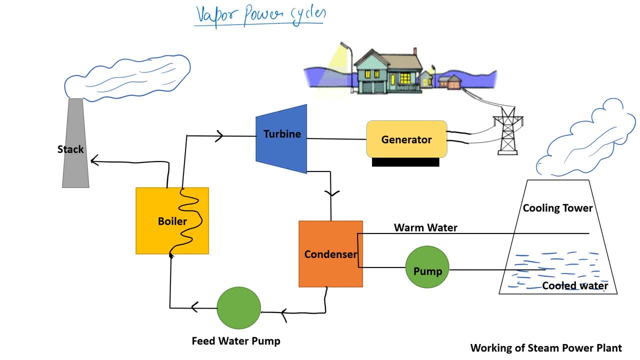 Vapor power cycle. In the vapor power cycle, the working fluid has a total of two components. There are two phases, Which are liquid and vapor. Half of the cycle will be of liquid and the other half of the cycle will be of vapor. 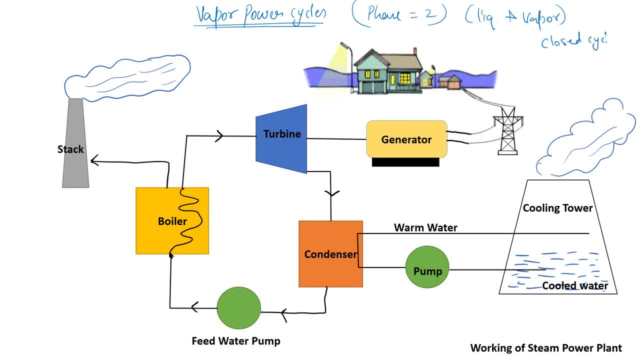 And what kind of cycle is this? This is a closed cycle. Boiler to turbine, turbine to condenser, condenser to feed water pump and feed water pump to boiler. In this way, the cycle keeps recirculating, So this is a closed cycle. 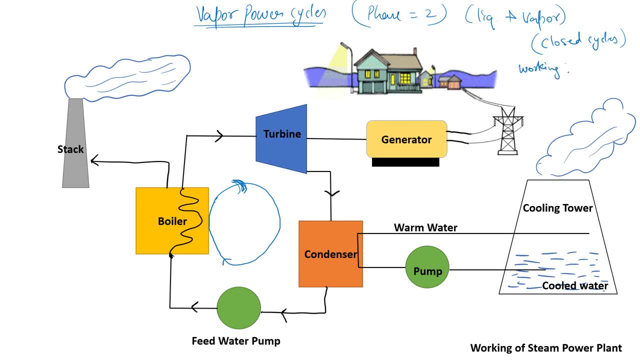 And the working fluid. in it, Working fluid, Water- is being used. That is why the name of this power plant is steam power plant: Because water is being used in the working fluid. Let's understand its working principle: Whenever the working fluid comes out of the condenser, it is of liquid nature. 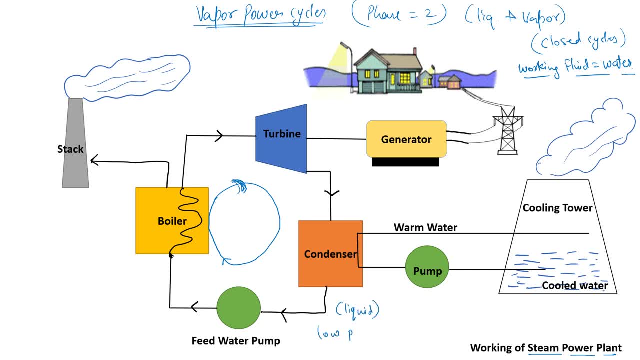 And here it is: in low pressure. Low pressure is liquid. Liquid enters the feed water pump. What is the work of the water pump? Increase the pressure. When the working fluid comes out of the water pump, its pressure will increase. If we convert low pressure into high pressure, then we will have to supply some work in this pump. 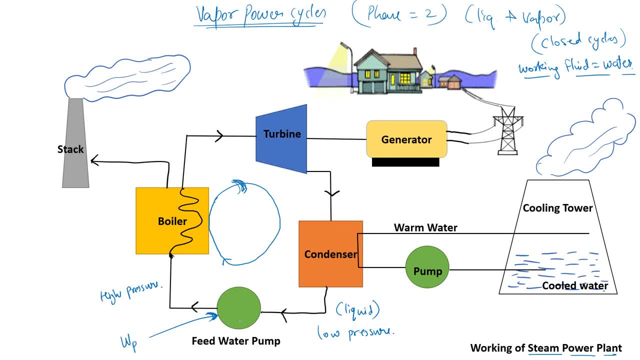 So this is WP. WP amount of work is supplied in the water pump. This increases the pressure of the liquid. So here we have a boiler from the condenser to the water pump and a boiler from the water pump. What is the phase in the half cycle? 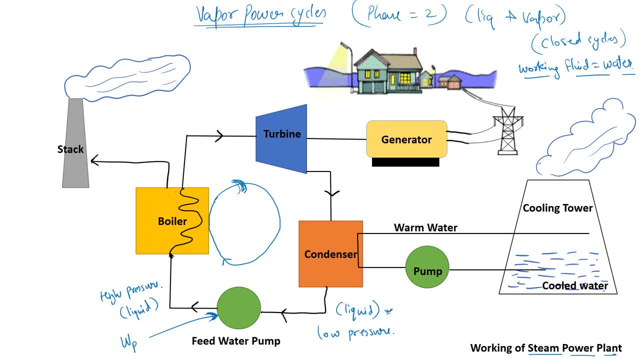 It is a liquid phase. Now see boiler. When the liquid comes out of the boiler, its phase will change. It will be in the vapor phase. Pressure will remain the same. The same pressure will remain here. Suppose this is 1.. 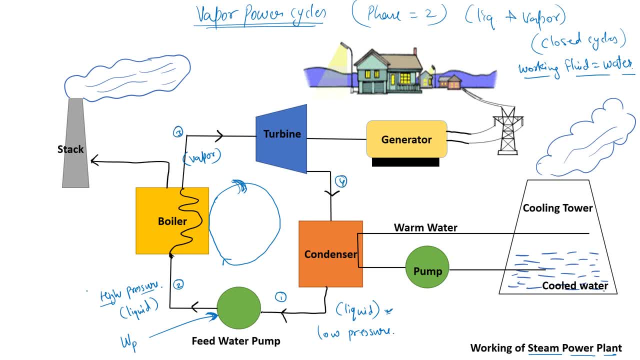 This is 2.. This is 3. And this is 4.. So P2 is the same, P2 is equal to P3.. The phase transformation is happening at constant pressure. We will add heat to the liquid Only then it will go to the vapor phase. 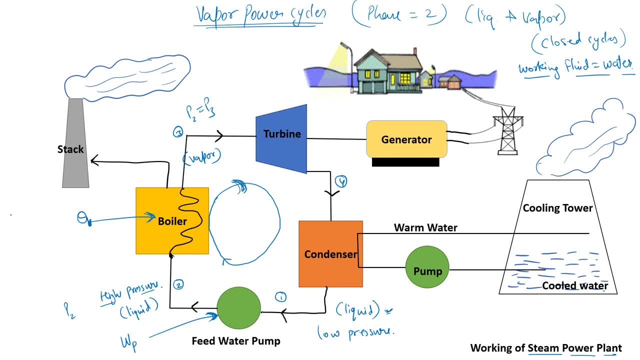 Now in the boiler we have to supply heat to QL. Now we supply this heat through coal or through nuclear fuel. If we are using coal in the fuel, then we will call it thermal power plant. If we are using nuclear fuel, then we will call it nuclear power plant. 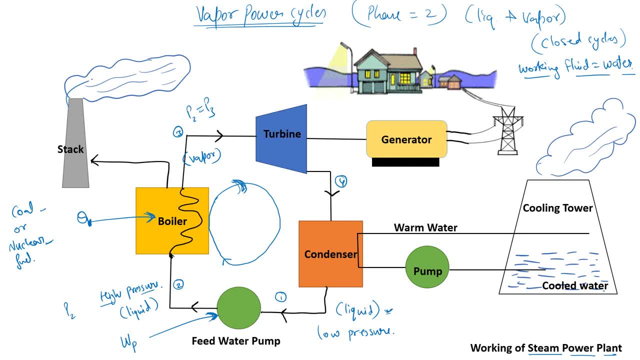 From here heat is being supplied to the boiler and flue gases are coming out from here. Flue gases are coming out: CO2, NO2, SO2.. Like this. Now see boiler. We have supplied heat to the boiler, So what did the water pump do? 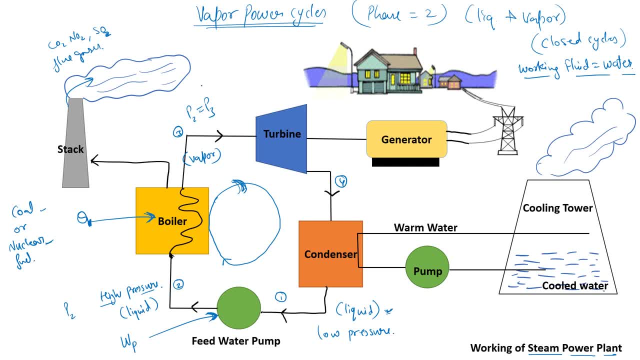 It increased the pressure. What did the boiler do? It increased the temperature. So high pressure and high temperature. If it is vapor, then we can also call it steam, Because the working fluid is water. So high pressure, high temperature and steam will come in contact with the turbine. 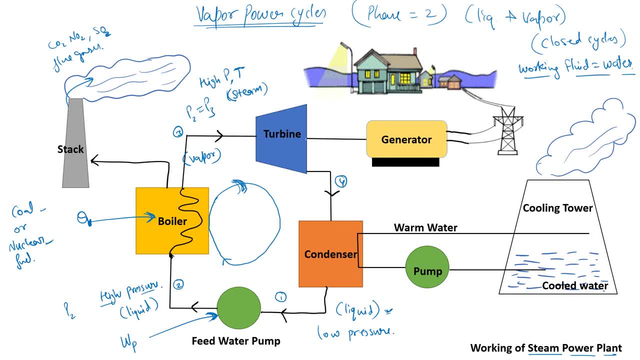 There are many blades in the turbine. They rotate And those blades are connected instead of shaft And this shaft goes inside the generator. So inside the generator, this is the rotating shaft. So what is the work of the generator? To convert mechanical energy into electrical energy. 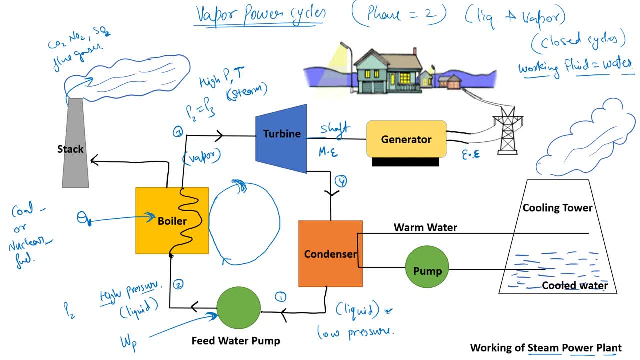 In electrical energy. So in this way we generate electricity Through which? Through these fuels- Coal and nuclear fuel- Because they have chemical energy. See here in which chemical energy was converted: It was converted into thermal energy, Then thermal energy was converted into mechanical energy. 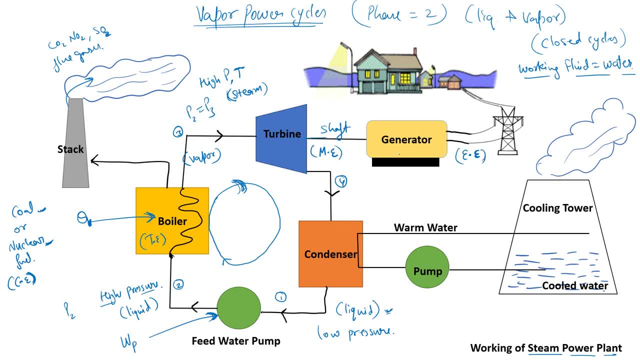 Mechanical energy was further converted into electrical energy. In this way, we are converting energy, Okay, So you see when the working fluid is coming out of the turbine, So what will be its nature? This will also come out as steam. Okay, Because what has the turbine done? 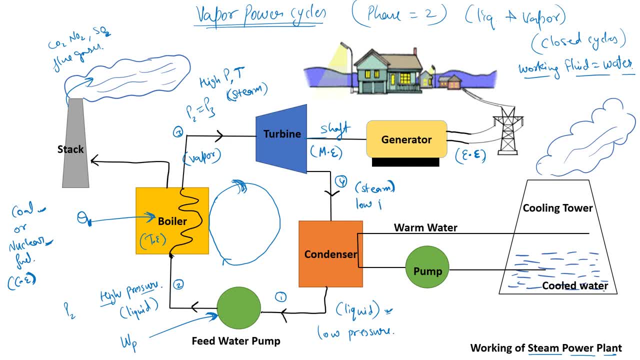 It has reduced the pressure only. Okay, It was high pressure, It was converted into low pressure. It was converted into low pressure. Okay, When low pressure steam is going inside the condenser? Okay, So what is the work of the condenser? 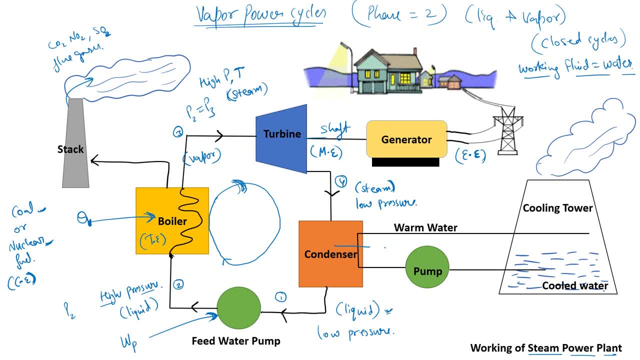 The work of the condenser is to remove latent heat. It is rejecting heat, Okay. What is the work of the condenser? It is rejecting heat from steam. Okay, When we will remove latent heat from steam, Then its phase transformation will take place. 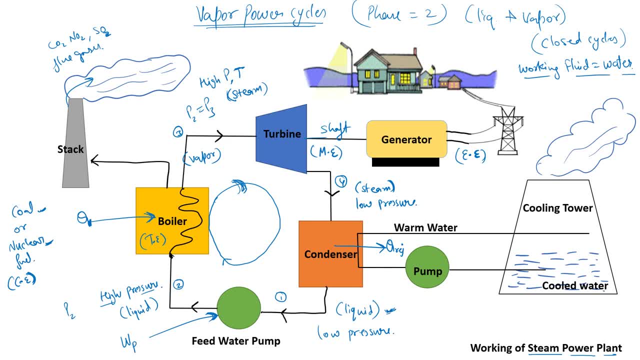 And it will be converted into what again? It will be converted into liquid. Okay, This is the cooling tower. In the cooling tower- see here- there is cooled water. In this way, water is flowing, Okay. So see here when the cooled water is coming in contact with the condenser. 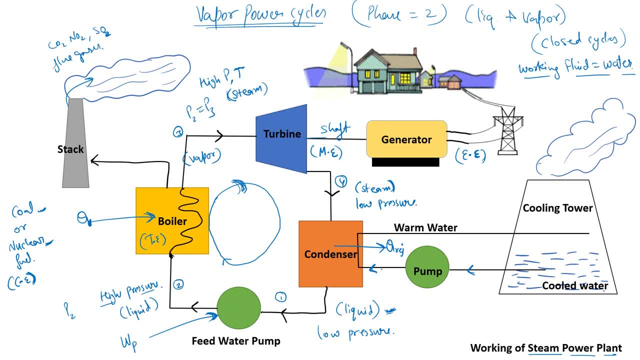 And what is there in the condenser? There is steam. Okay, So from the steam, this cooled water will exchange heat in each other. Okay, It is also called heat exchanger. Heat will be exchanged in each other And this cooled water will be converted into what? 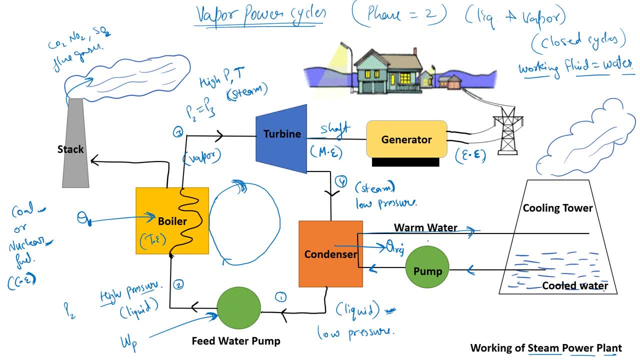 It will be converted into warm water. Okay So, in this way, heat is being rejected. Okay, So, this is our complete working principle. So see, here in the feed water pump, we have supplied work. In the boiler, we have supplied heat, We have got work from the turbine. 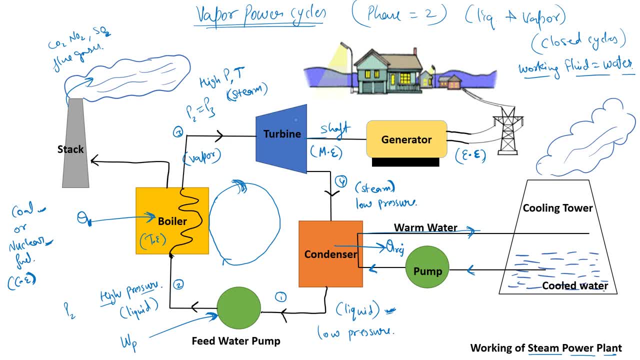 This is WP. Okay, And heat is being rejected from the condenser. Okay, So in this way, the whole cycle is there. Okay, So you understood how we are generating electrical energy. Okay, So this was our steam power plant. Okay. 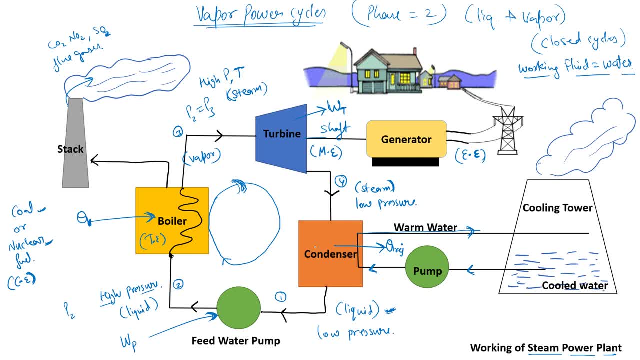 Now we call this cycle as Rankine cycle, Okay, Which we are going to discuss in today's video. Okay, So this is our steam power plant. Okay, So this is our steam power plant. Okay, Now we are going to discuss this cycle in today's video. 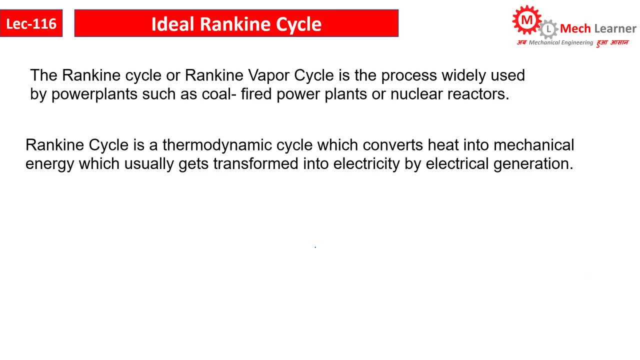 Okay, So we are going to discuss this cycle in today's video. Okay, So let us start Ideal Rankine cycle. Okay, In next video we will talk about actual Rankine Cycle. Let us discuss the ideal Rankine Cycle first. 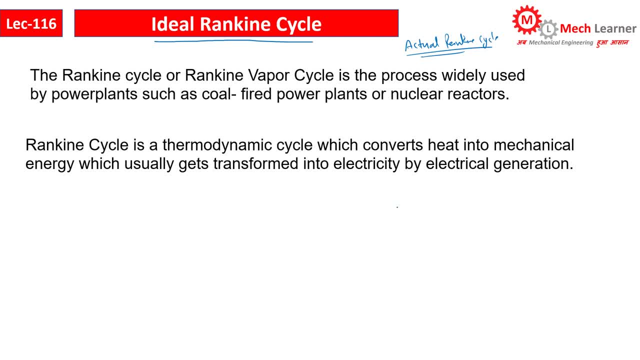 Okay, The Rankine cycle and Rankine vapour cycle is the process widely used by power plants such as the coal fired power plants and nuclear reactors. Okay, Mean in the Neuclear Power Plant and the coal powered Plants, we will use the Rankine. 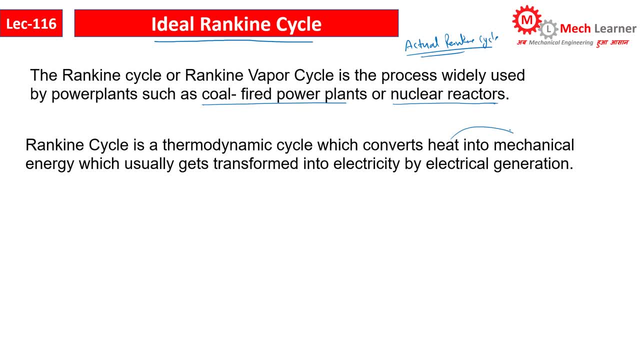 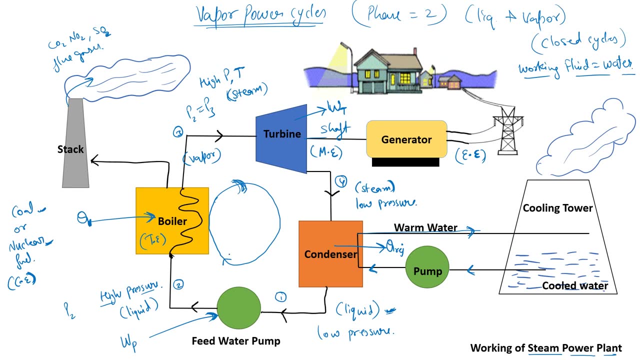 Racinic cycle Okay, which converts heat into mechanical energy and then it is further transferred to electricity by the help of generators. So this is the entire Rankine cycle. Energy is converted in the Rankine cycle. Chemical energy is converted into thermal energy. 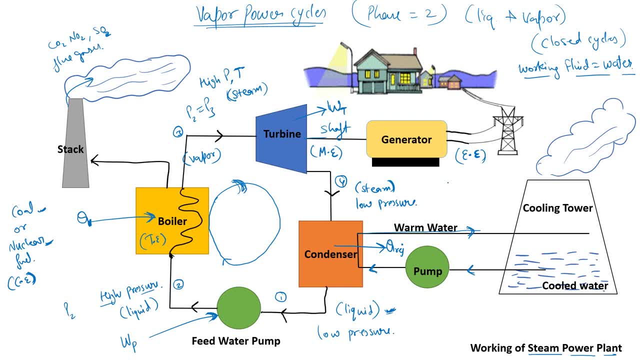 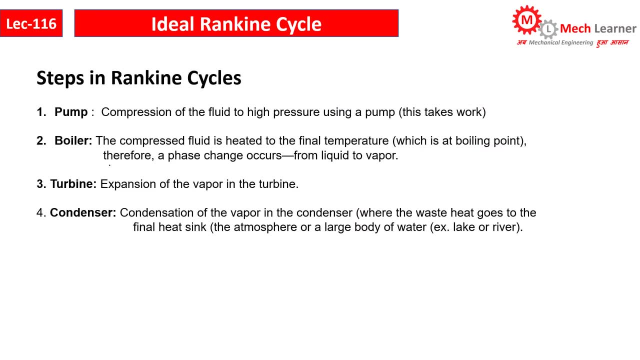 thermal energy into mechanical energy and mechanical energy into electrical energy. So this entire cycle is known as the Rankine cycle. Next let's discuss the steps of the Rankine cycle. There are four steps in the Rankine cycle: Pump, Boiler, Turbine, Condenser. 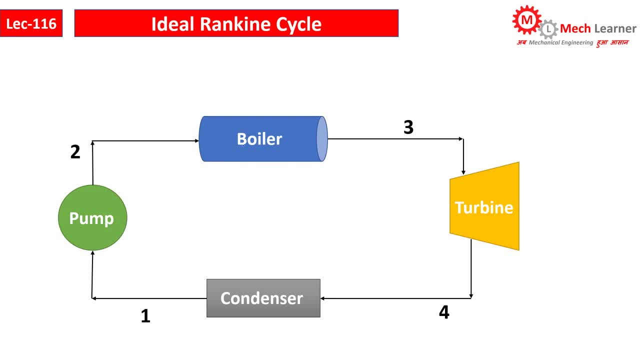 So this is the arrangement of the Rankine cycle: Boiler, Boiler Turbine, Turbine Condenser, Condenser Pump. This is the Rankine cycle. Look at the direction of the cycle. It has a clockwise direction. 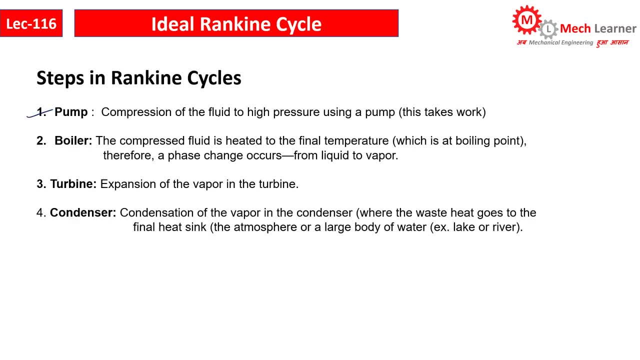 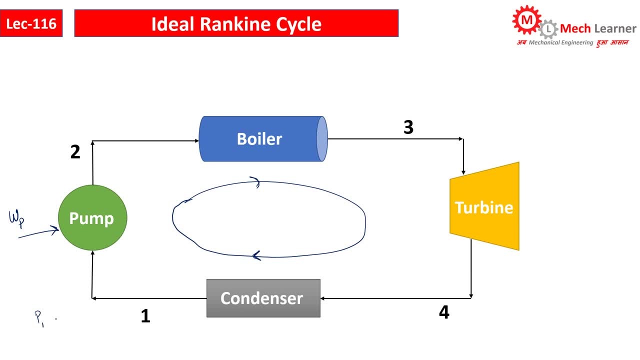 The first step is the pump. What is the pump doing? It increases the pressure of the fluid In which we have to supply work to the pump. Wp: Suppose here the pressure is P1, the temperature is T1 and the enthalpy is 1.. 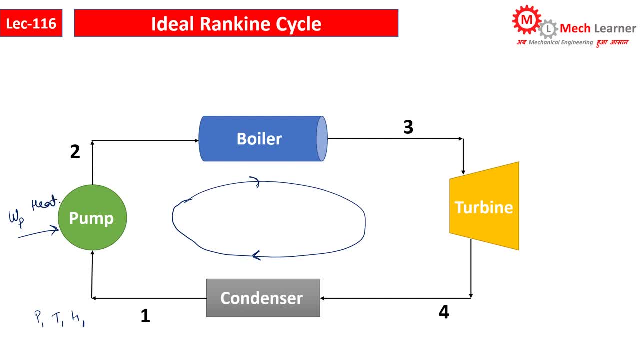 So this is the heat pump. In the heat pump the pressure will also increase and the temperature will also increase. So here the temperature is T2, the pressure is P2 and the enthalpy is H2.. The pressure is increasing, so P2 is greater than P1.. 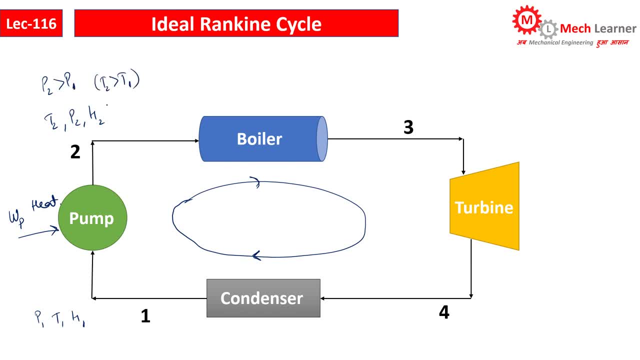 And T2 is greater than T1.. And the working fluid here is of liquid nature. This is saturated liquid. Saturated liquid Now, saturated liquid, is going into the boiler. Now, if we supply heat, This is Q1.. We have supplied heat in Q1.. 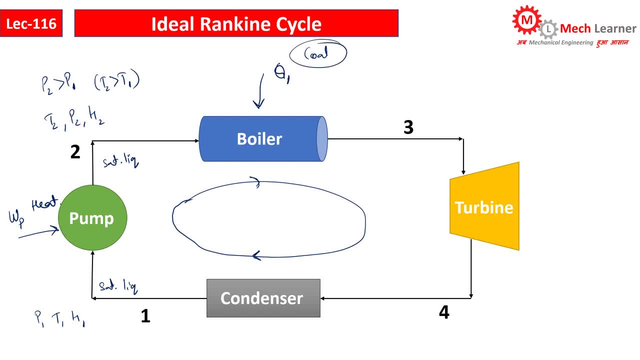 Where is the heat being supplied from? It is being supplied from the coil. Now the heat is being supplied And this is saturated liquid. When we add heat in saturated liquid, it will be converted into saturated vapour, And if we add more heat, it can be superheated vapour. 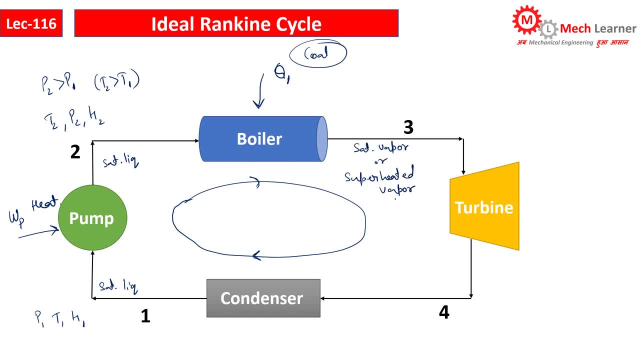 Superheated vapour, And if the working fluid is water, then we will call it steam. Okay, So here the pressure will be P3, the temperature will be T3. The enthalpy will be H3.. Okay, 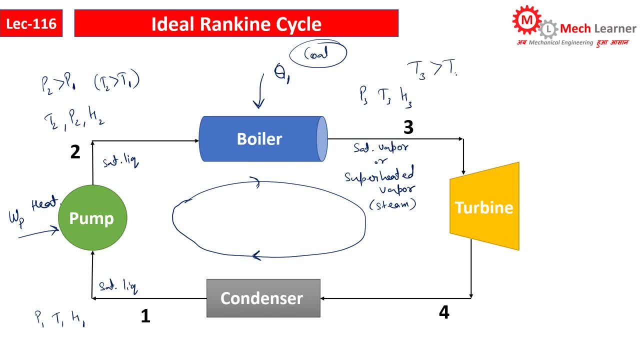 So if we are supplying heat in the boiler, then the temperature will increase. So T3 is greater than T2.. Okay, But the pressure will remain the same. P2 is equal to P3.. Okay Now, high pressure, high temperature steam. 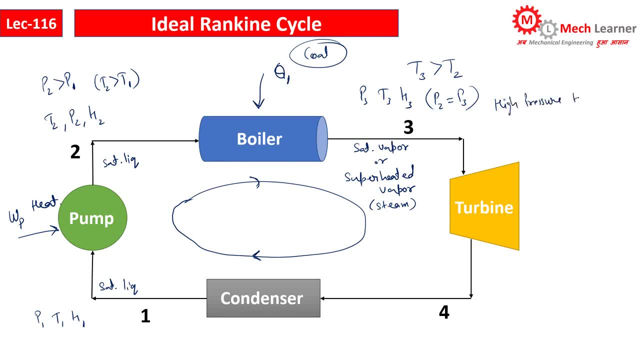 High pressure. The pressure pump has increased High pressure And the temperature has been increased by the boiler. High pressure, high temperature steam will go through the turbine, Okay, So this will be converted into low pressure steam, Okay, And the temperature will also be reduced. 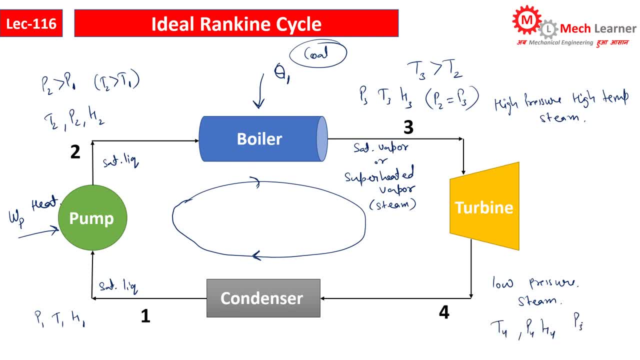 So this is T4, P4 and enthalpy is H4. Okay, So P3 is greater than P4.. And the temperature is also reduced, So T3 is greater than T4.. Okay, The job of the turbine is to produce the work. 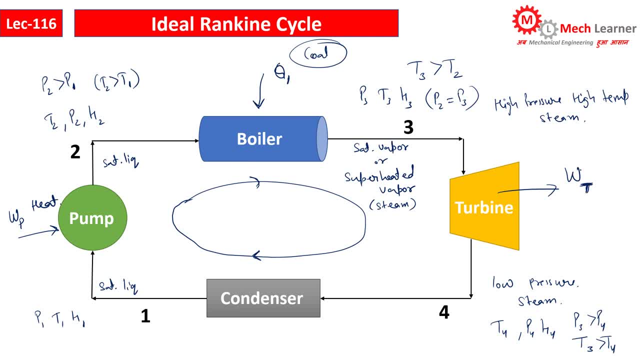 So this is turbine work. Okay, So here again, low pressure steam In which it is entering. It will enter in the condenser. What will be the work of the condenser? The condenser will remove the latent heat from the low pressure steam. 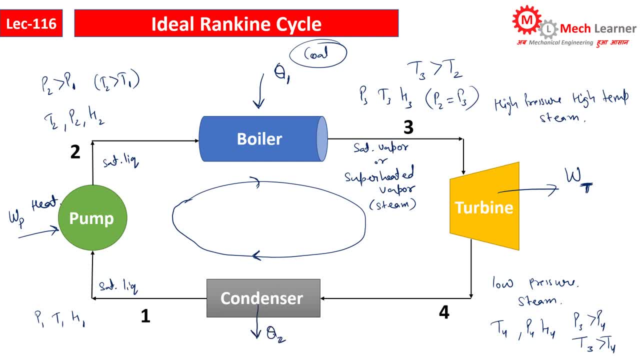 Okay, When it will remove the latent heat, then the vapor will be converted into liquid. Okay, Condenser is rejecting the heat Boiler. We are supplying heat in the boiler. The turbine is producing the work. We are supplying work in the pump. 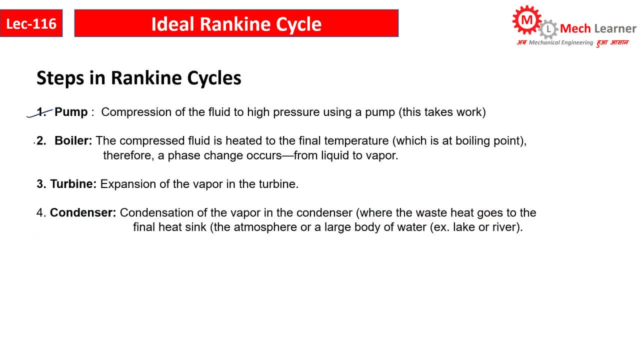 So these are the total four steps of the Rankine cycles. Okay, Pump Compression of the fluid to high pressure using a pump. Okay, We have supplied work in the pump. This is WP. What are we doing in the boiler? 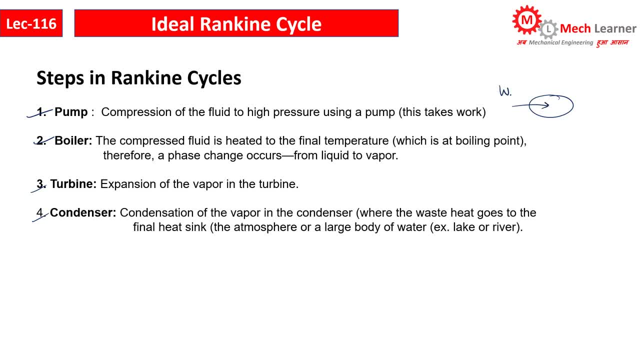 We are supplying heat. Okay, Compressed fluid is heated to the final temperature. Okay, So this is the final temperature. Okay, So this is the final temperature. Okay, So this is the final temperature. So this is the final temperature. 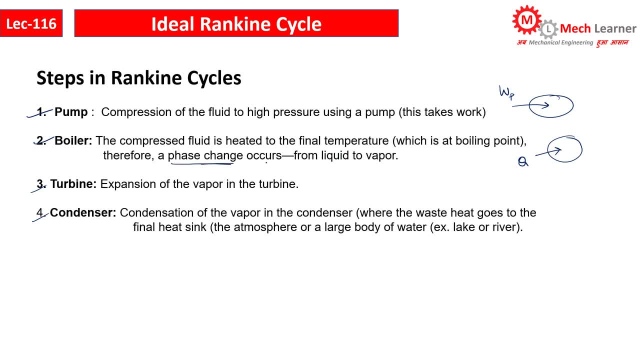 Okay, As per rankine cycles quickly. the próxima phase is heated to the final temperature and even the phase is being changed in the boiler. Liquid is being converted into the vapor. Work is being done in the turbine. This is WP. Okay. 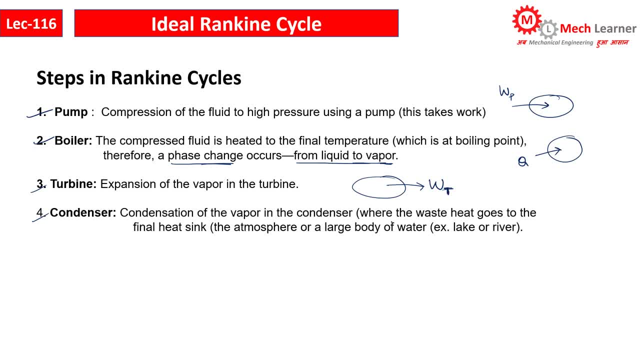 This is turbine work Condenser. What is condenser doing? It is rejecting heat. Okay, It will either eliminate heat in the cooling tower or in the lake or river. Okay, So this is rejecting heat. Still, some phase transformation is taking place in it. 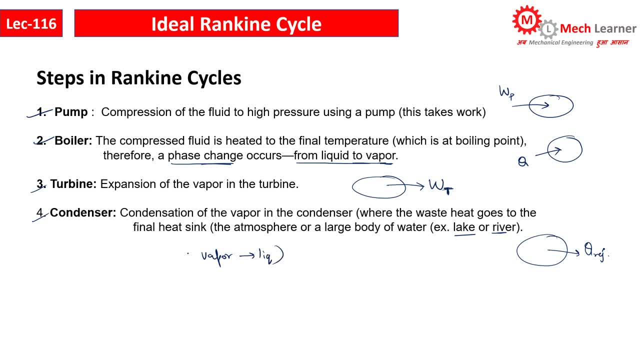 Where is the vapor converted? It is converted in the liquid. Okay, So there is phase transformation in the condenser and phase transformation in the boiler. So these are the four steps of the Rankine cycle. Now let's assume some assumptions of the Rankine cycle. 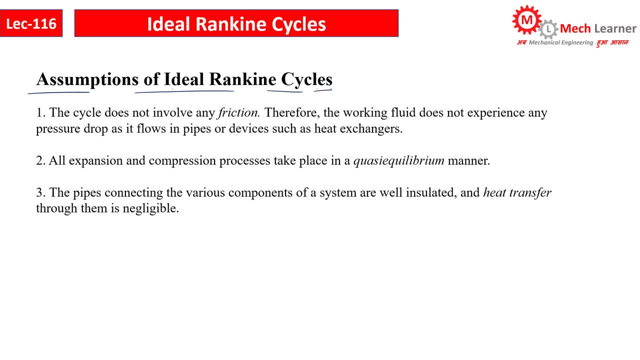 There are assumptions of the ideal Rankine cycle. It will be opposite to the actual Rankine cycle. The first assumption is that the cycle does not involve any friction. The friction in this cycle is assumed to be zero, Due to which the working fluid does not experience any pressure drop as it flows in pipes or devices such as heat exchangers. 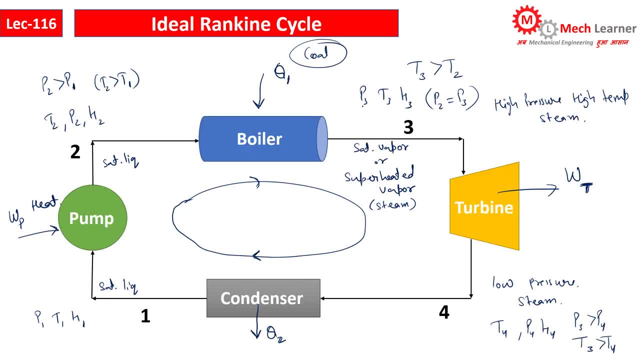 Here there was P2 pressure and here there was P3 pressure. So we supplied heat in the boiler Pressure is the same: P2 is equal to P3.. Similarly, here the pressure is P4 and here the pressure is P1.. 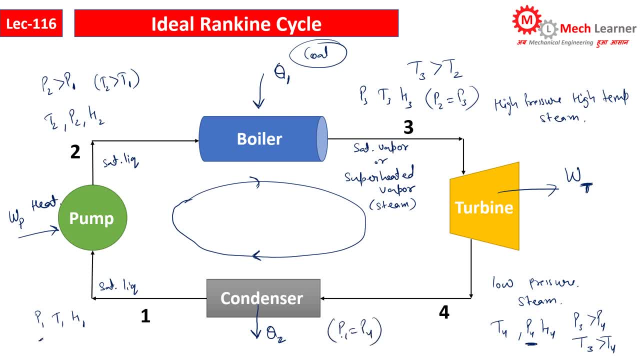 So P1 is equal to P4. We are rejecting heat at constant pressure. Pressure is constant because the friction in this pipe is zero. If there is friction in the pipe, then these two pressures will be present. They will not be equal to each other. 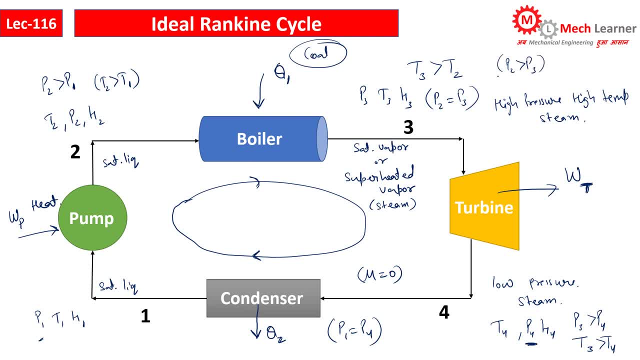 In that case P2 is greater than P3. Because when the working fluid flows in it and there is friction, then due to friction there will be some pressure drop. This will be discussed in the actual Rankine cycle, But if it is the ideal Rankine cycle, then let's assume that the friction is zero. 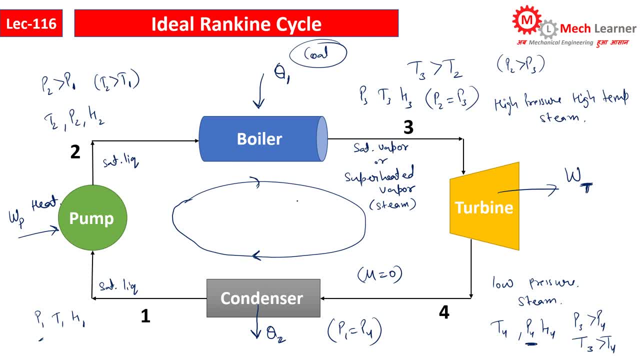 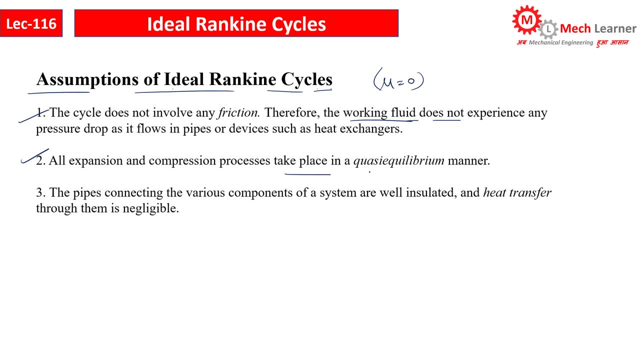 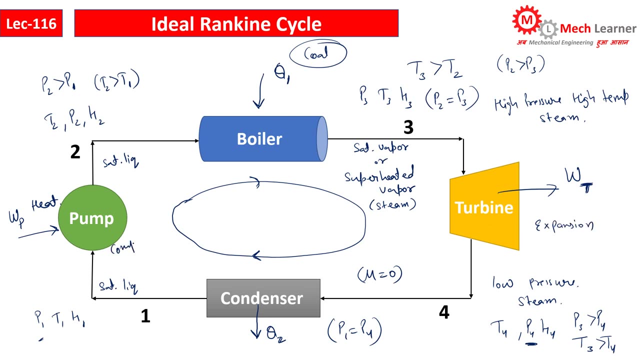 Due to which the pressure in the boiler and condenser will be constant. Next assumption: Expansion and compression process take place in a quasi-equilibrium manner. Expansion takes place in a turbine. Expansion takes place in a turbine. Compression takes place in a pump. 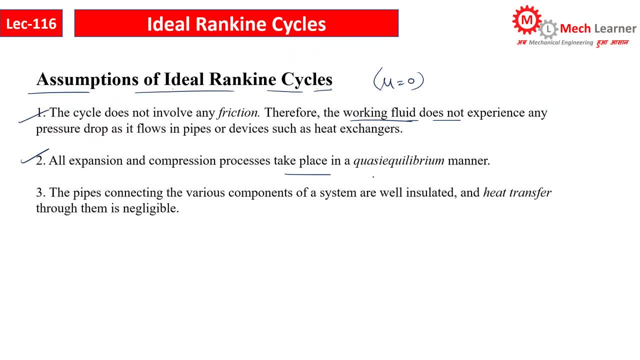 These two processes are quasi-equilibrium. Quasi-equilibrium means that the net force is zero, The chemical reaction is zero, We will supply heat at a constant temperature. It is a reversible and slow process. This is the assumption. The third assumption is that the various components of the pipe connecting 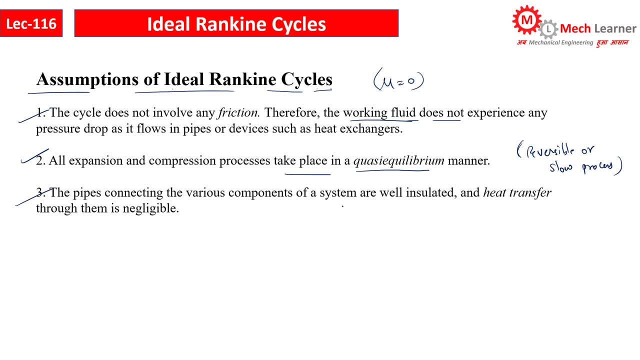 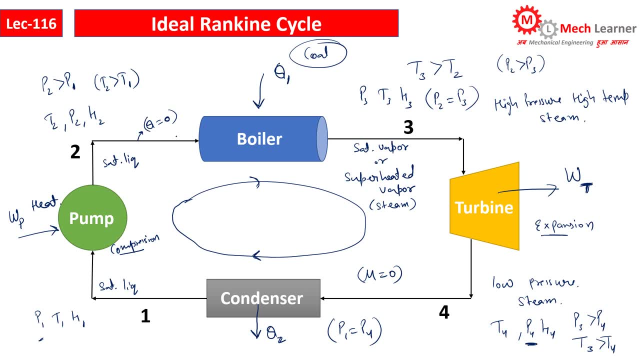 the various components of the systems are well insulated and heat transfer through them is a negligible. The heat transfer from this pipe to the system surrounding is zero. We have used an insulated pipe. This turbine is also insulated, But in the actual Rankine cycle. 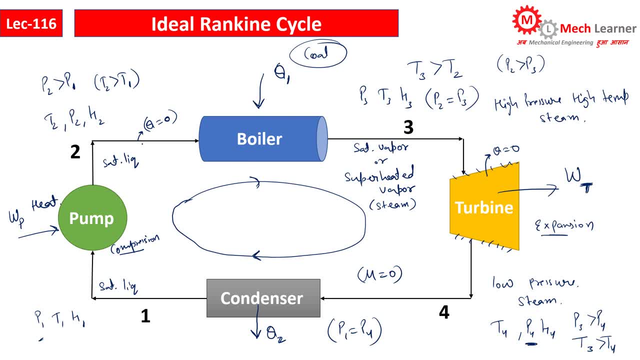 some amount of heat will also be transferred to the system surrounding. So this entire pipe is insulated. This pump is also insulated. So here we have discussed the assumptions of the Rankine cycle. Now we will draw the equations on these four devices. 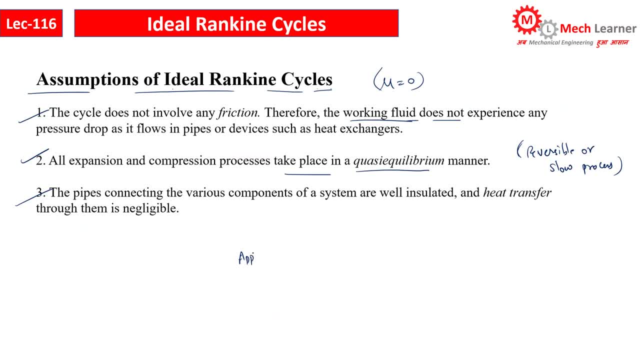 with the help of Steady Flow Energy Equations, Let's apply it here. Steady Flow Energy Equation: Inlet energy is equal to outlet energy, So Q in plus enthalpy, in plus kinetic energy. inlet plus potential energy in plus W in. 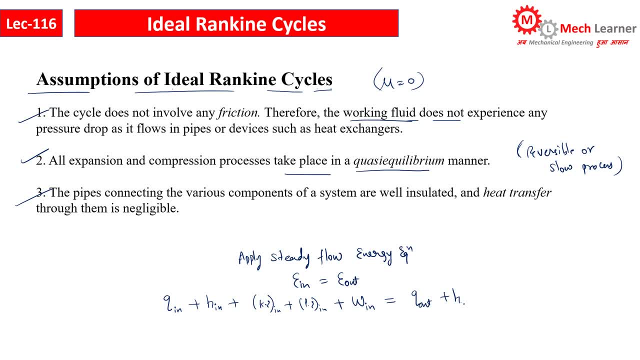 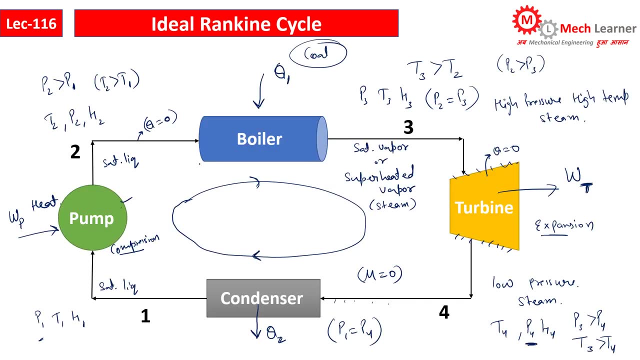 is equal to Q out, H out plus W out, plus kinetic energy outlet plus potential energy out. So this is our Steady Flow Energy Equation. Now look at these four devices: pump, boiler, turbine, condenser. These are all Steady Flow Devices. 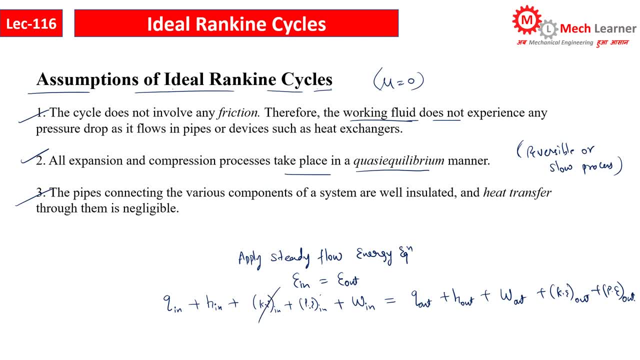 So in Steady Flow Devices the change in kinetic energy and potential energy is neglected, So it will be cancelled out. So here let's write four assumptions: Boiler, Compressor, Condenser Turbine and Heat Pump. 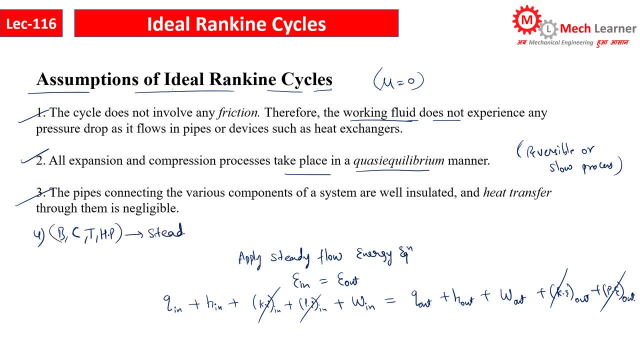 These four are our Steady Flow Devices. They are Steady Flow Devices, So change in kinetic energy and change in potential energy are neglected. So this is our Energy Equation. Let's write the Energy Equation here: Q in plus H in. 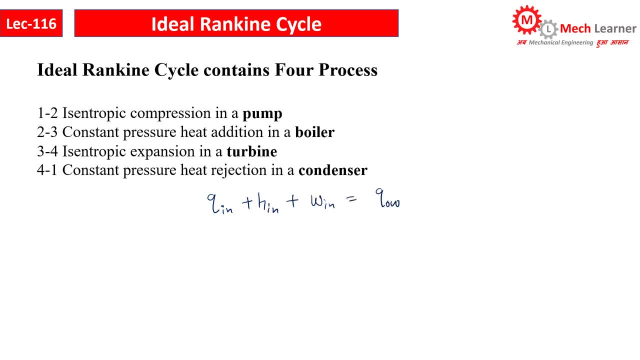 plus W in is equal to Q out plus this equation we will apply on all these devices In an ideal Rankine cycle. there are four processes in total. The first process is Icentropic Compression in Pump. This is 1 and this is the 2nd. 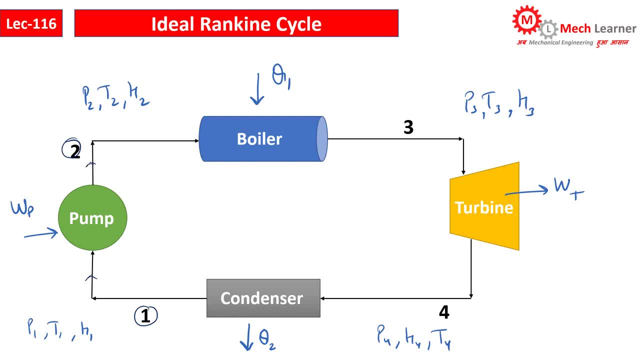 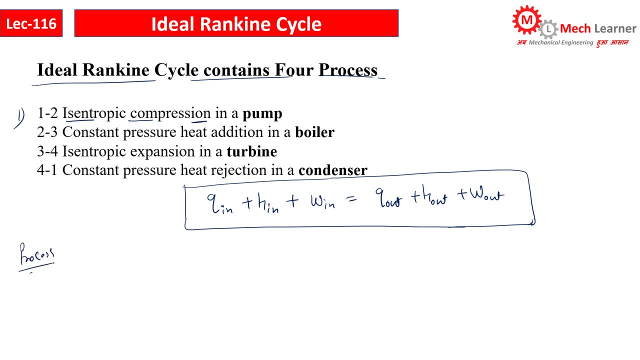 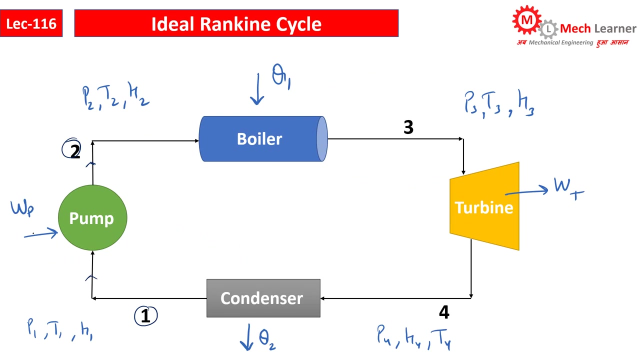 The first, when the working fluid is moving. the name of this process is isentropic compression process, process 1 to 2: isentropic compression process because pressure increase of fluid and we are supplying work from above. so see, here this pump is insulated, so neither heat energy is being added nor heat energy is being removed. 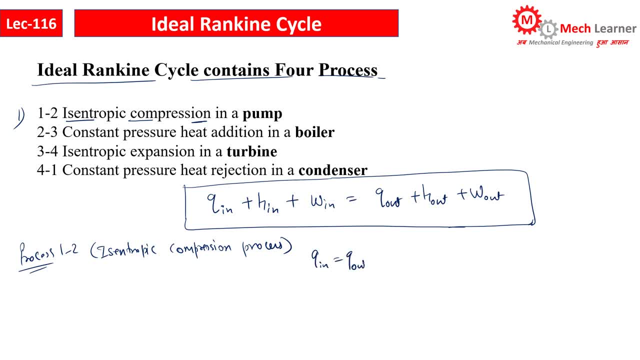 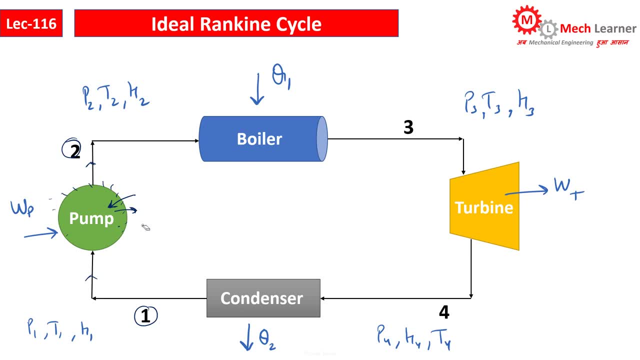 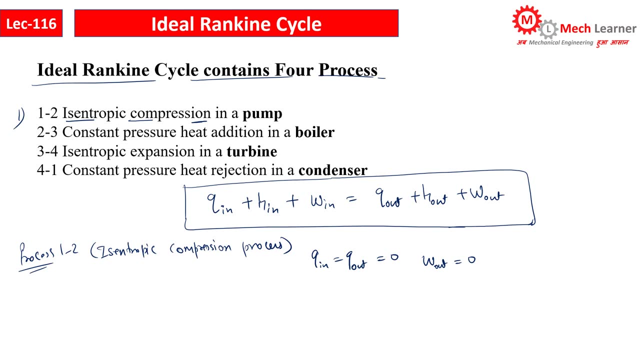 so Q in and Q out in the case of pump is 0 and we are supplying work in the pump. work done by the pump is 0 and we are not getting work from pump, so W out is also 0. so this is H enthalpy. inlet. inlet enthalpy is 1, so we are denoting it from H1. 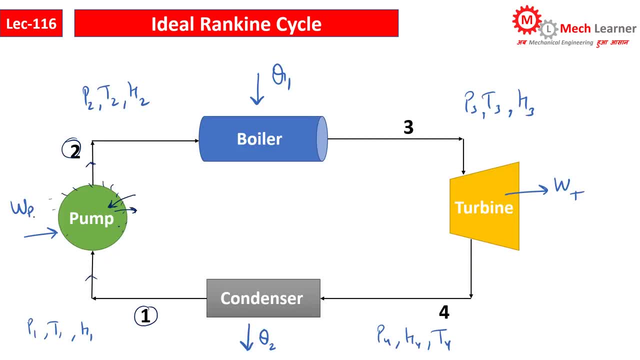 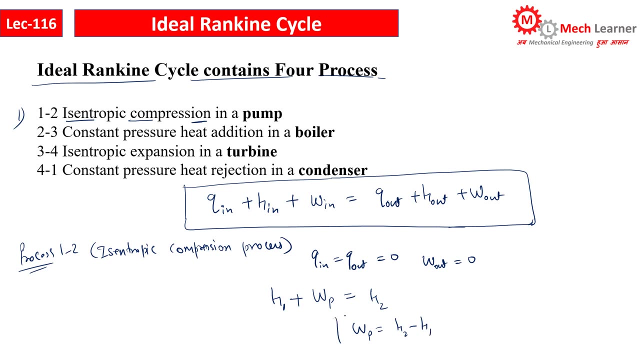 H1 plus inlet work is Wp. Wp is equal to outlet heat is 0, H out Wp is equal to outlet heat is 0. here outlet enthalpy is second, which means H2, so pump work is done. H2-H1, this is pump work. 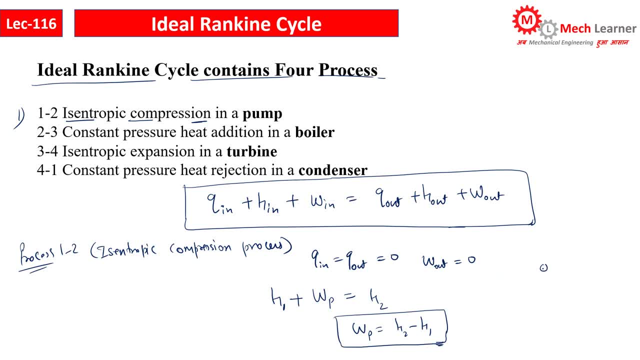 and we can also write: as this is open system, if pump is open system, then we are applying this formula in open system. so this is V and this is P2-P1. this is pump work. We can calculate like this and also like this. So the first process is isentropic compression. 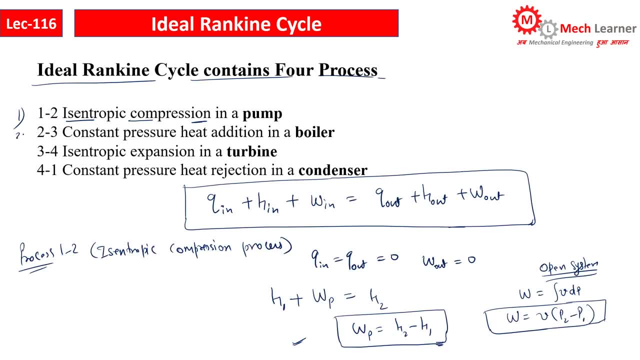 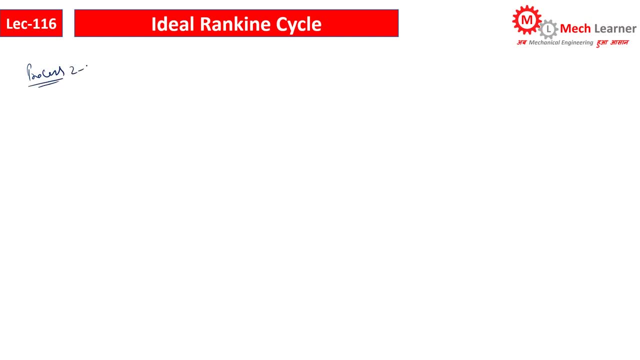 Compression because we are supplying work inside the pump. Next second process is 2-3 constant pressure heat addition in a boiler Process 2-3. This is isobaric heat addition process, So we are adding heat inside the boiler. Are we getting work from the boiler? No, 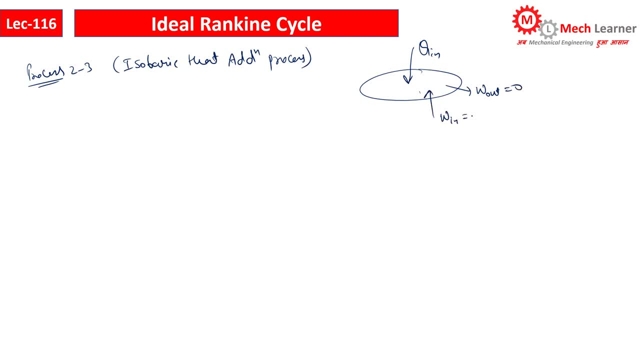 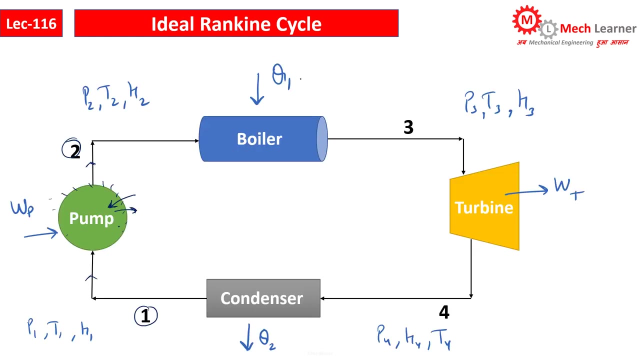 So Wout is 0. Are we getting work from the boiler? No, So Win is 0. And this boiler is insulated, So the heat transfer is negligible, So Qout is also 0. Now look at the energy equation. This will be Qin. Qin is equal to Q1. 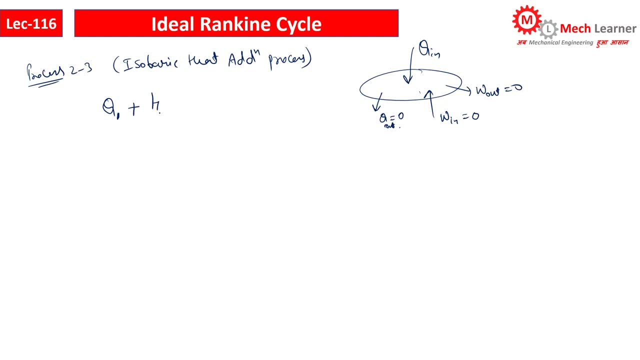 This is Q1, Plus inlet enthalpy is H2, The enthalpy entering the boiler Is H2 And out is H3. The rest is 0. So this is Q1. Q1 is equal to H3 minus H2. This is our heat supply in boiler. 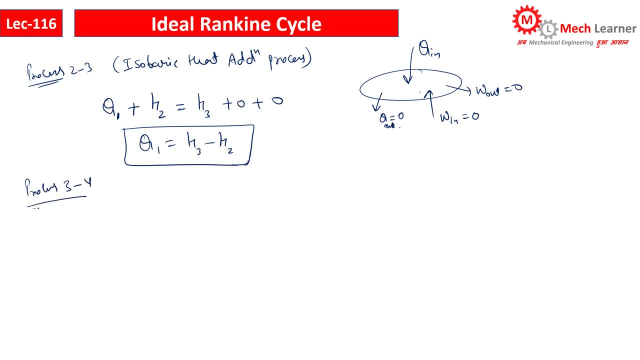 Next process: 3-4. The name of this process is 3-4. Third process is isentropic expansion in turbine. This is also isentropic process, Isentropic Expansion, Expansion process. So in this turbine We are getting the work. This is outlet work. 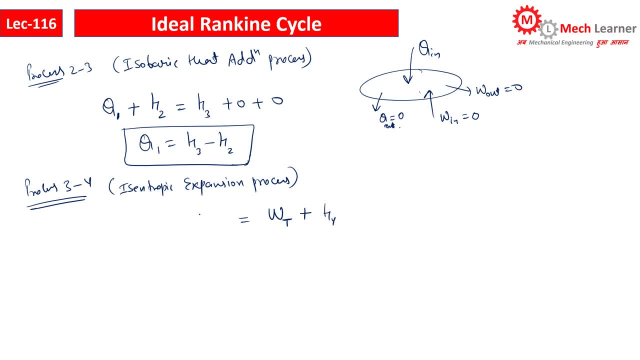 Wt. Outlet enthalpy is H4, Inlet enthalpy is H3. Rest is insulated turbine. So neither the heat is added nor removed. So turbine work is equal to H4. This is H3 minus H4. this is the turbine work. last process, process 4. 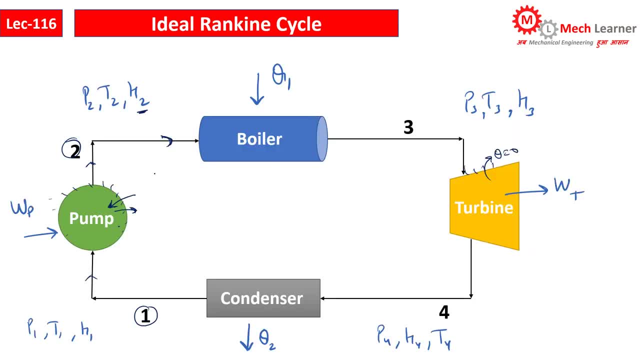 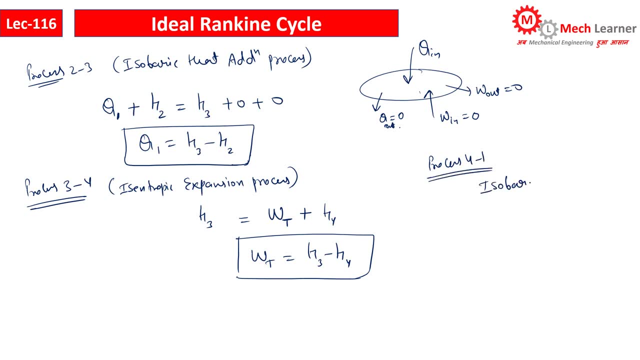 4-1. constant pressure heat rejection in a condenser process. 4-1. this is isobaric. isobaric heat rejection process. ok, in condenser, heat is being rejected. heat is being rejected. Q2 will come here. how much is the enthalpy H1? 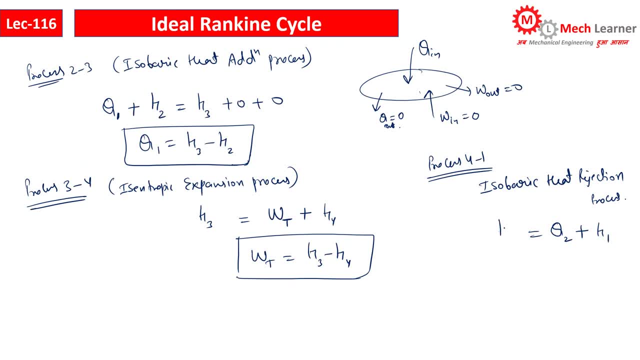 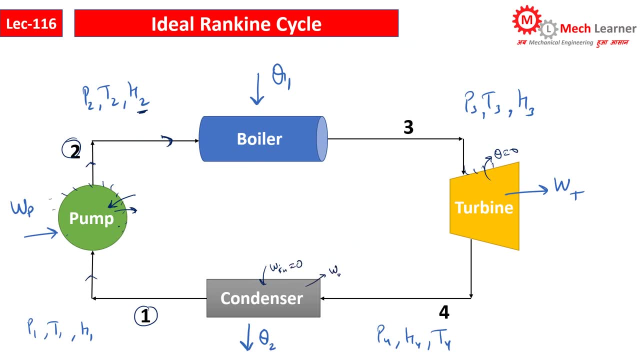 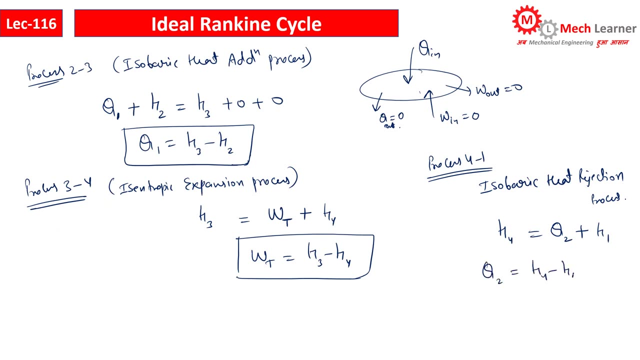 in inlet condenser. enthalpy is H4 rest. we don't supply work in condenser. we don't supply work and we don't get work. so outlet and inlet work is 0. Q2 is equal to H4-H1. this is heat rejection. 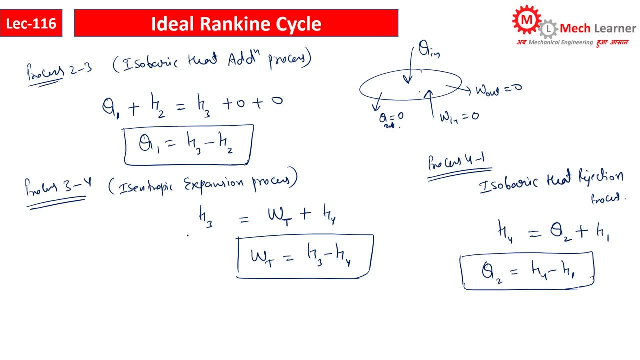 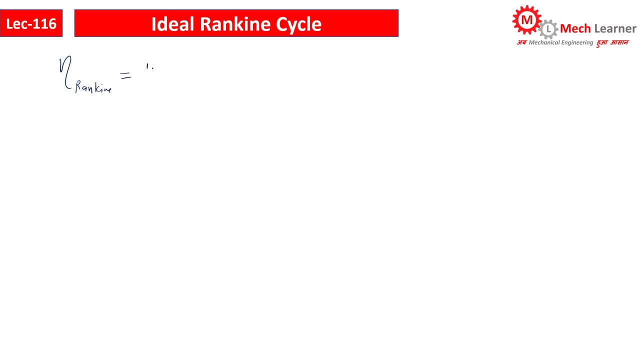 ok, now let's find the efficiency of this cycle. so efficiency of rankine cycle is equal to net work done divided by amount of heat supply. this is the expression of efficiency. now let's find the net work done with the help of first law of thermodynamics. 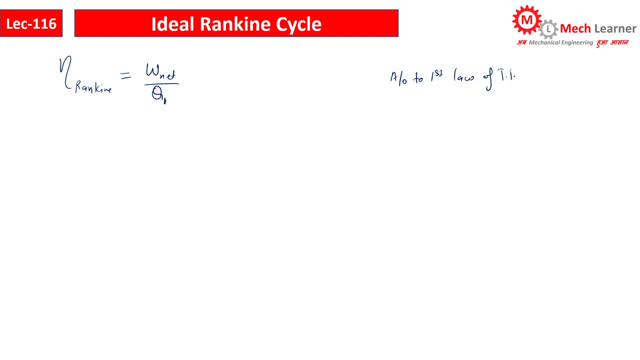 according to first law of thermodynamics. there are two expressions in this. if process is going on, then first law of thermodynamics is this: if cyclic process is there, cyclic process- then expression is net heat is equal to net work, so rankine cycle is a cyclic process. 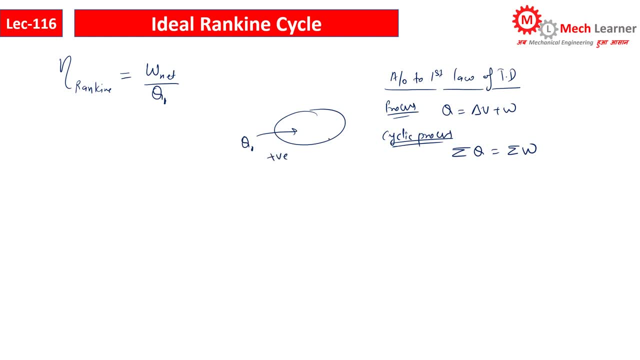 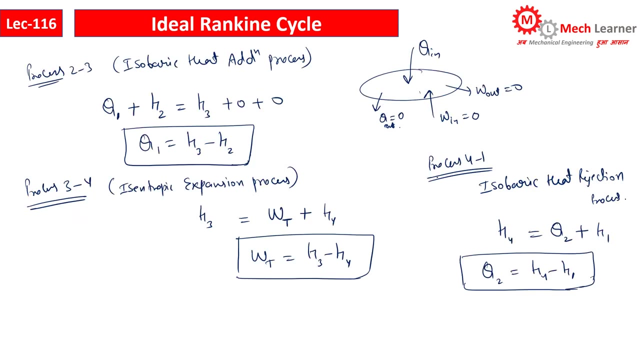 so let's see sign convention: whenever heat is supplied in system, then it is positive. if heat rejection is there, then it is negative. similarly, when we supply work in system, then this is negative and work done by the system is positive. so let's find net heat in this rankine cycle. 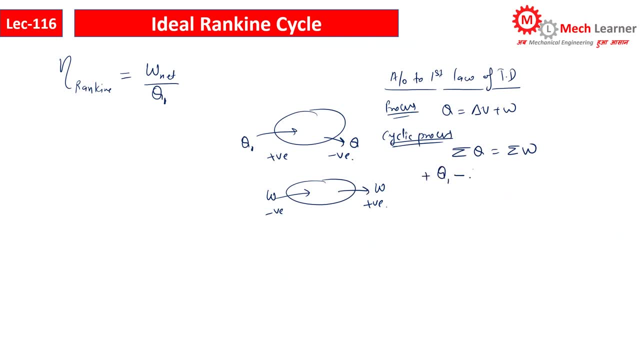 Q1. amount of heat is being added in this system, so heat supply is positive. so this is minus sign. minus Q2: work is being produced by turbine, so this is plus Wt and we are supplying work in this pump, so this is minus Wp. so here: 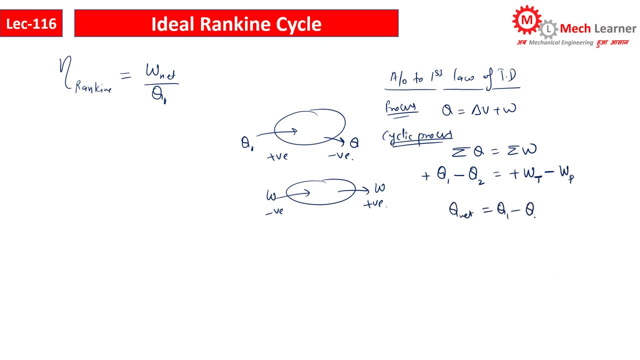 net heat is equal to Q1 minus Q2 and net work is equal to Wt minus Wp. so efficiency of rankine cycle is equal to Wt minus Wp divided by amount of heat supply. ok, turbine work. turbine work is equal to H3 minus H4. 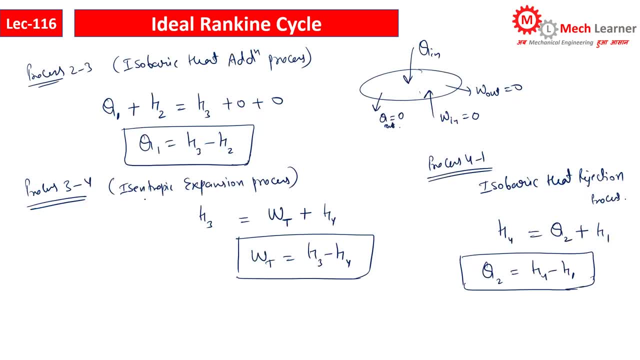 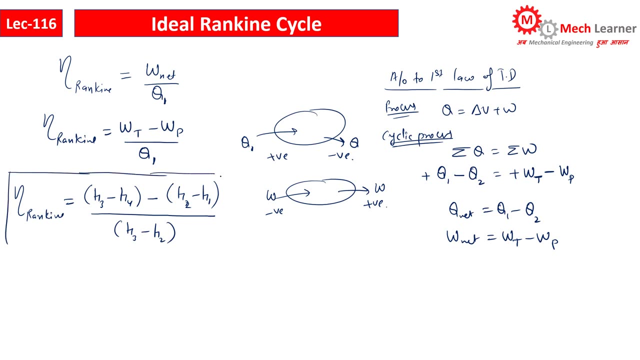 ok, pump work is equal to H2 minus H1. divided by amount of heat supply, that is equal to H3 minus H2. so this is our efficiency rankine cycle efficiency. when we will consider pump work, pump work is considered. let's take a case when we will not consider pump work. 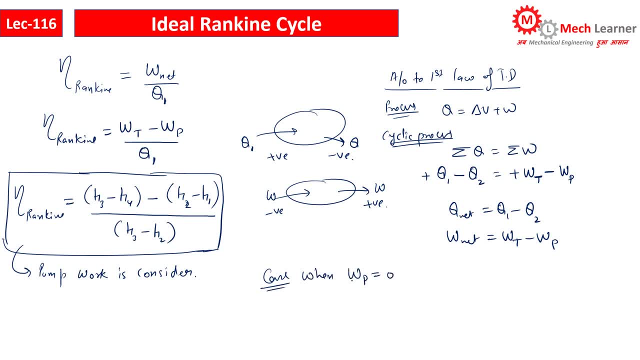 when, when pump work is zero. so efficiency of rankine cycle efficiency will be H3 minus H4, H3 minus H2, H3 minus H2. this will be efficiency, this efficiency. we call it like this: isentropic, isentropic, isentropic efficiency of. 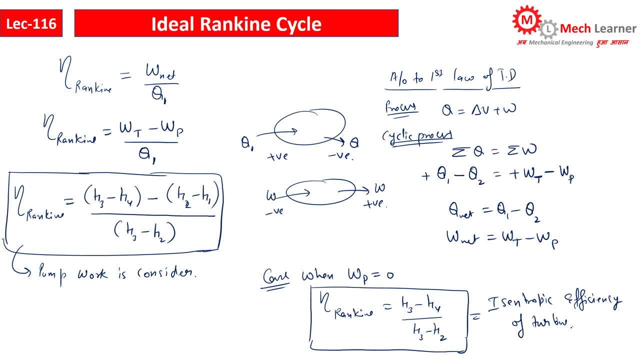 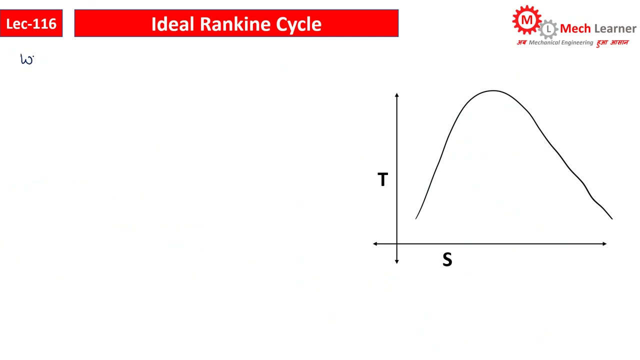 isentropic efficiency of turbine. this is special case. this is special case. this is special case because we assume that turbine work is greater than pump work, so difference will be Wt minus Wp. this is approximately equal to turbine work. so this is why this is why- 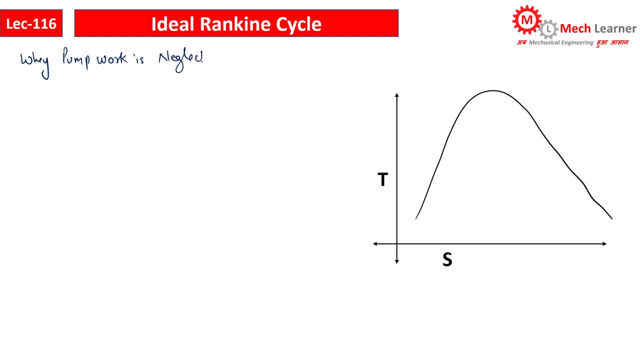 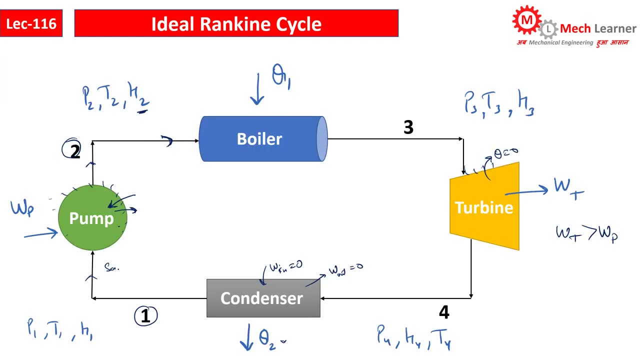 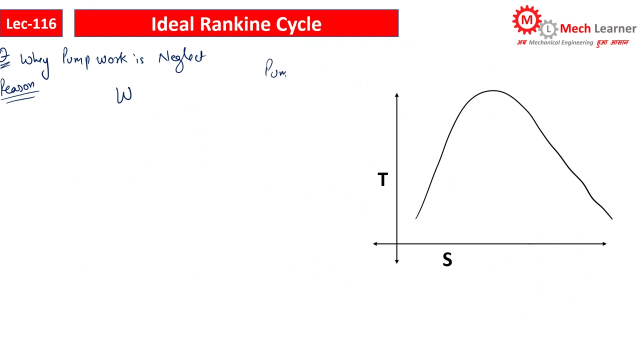 why pump work? pump work is neglect is neglect. reason we will understand reason we will understand. see, in pump the working fluid is entering saturated liquid and in turbine, working fluid enters saturated vapor. ok, This is open system. This is the expression of work in open system. 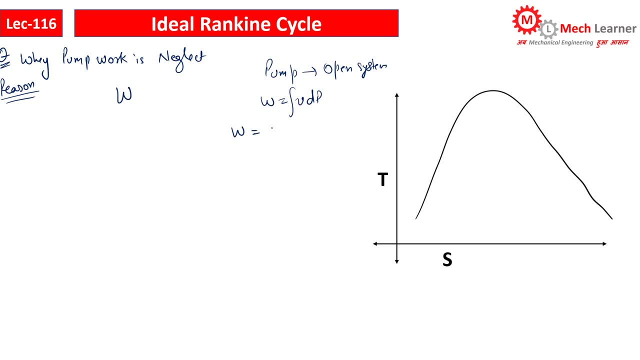 Work is equal to specific volume at saturated liquid, And this is P2 minus P1.. This is pump work. Similarly, turbine work will be specific volume at saturated vapor. So here Vg will come And that is pressure. Let's see once. 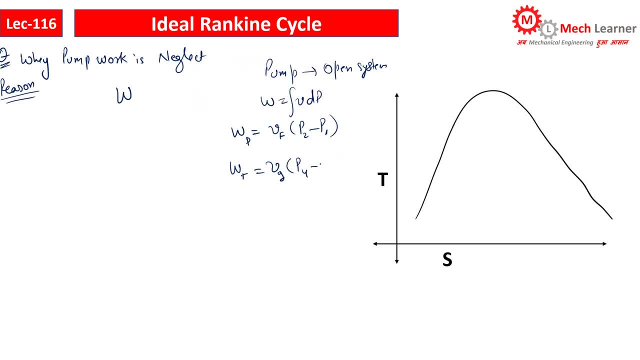 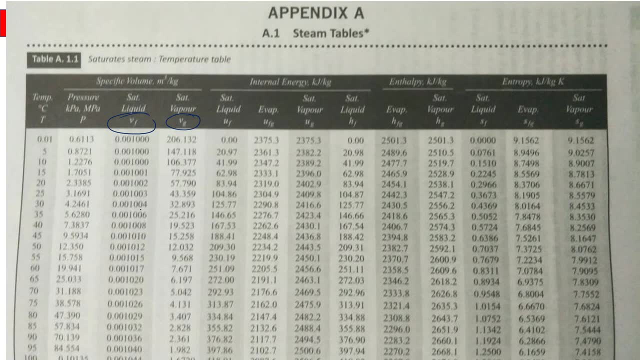 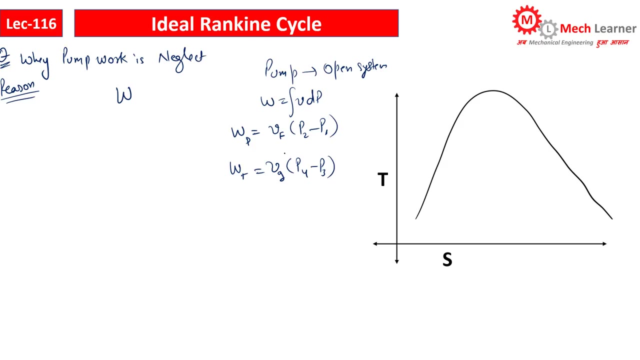 This is P4 minus P3.. P4 minus P3.. Look at the steam table. This is saturated liquid and this is saturated vapor. Compare Vg and Vf. Vf is a very small value: 0.001023. Specific volume at saturated vapor is much greater than specific volume at saturated liquid. 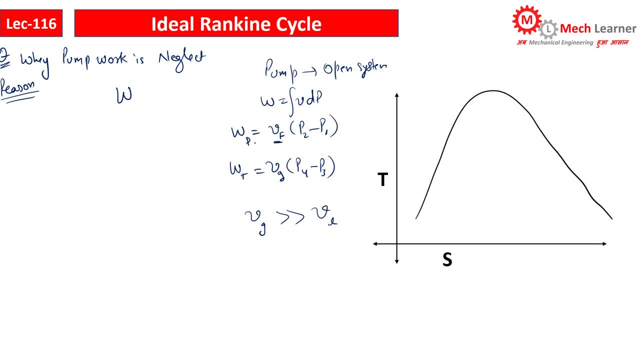 When we write the value of Vf here, Wp will come approximately near 0. That is why we neglect the pump work. So the reason for this is Vf is equal to P2 minus P1.. And the pump work. 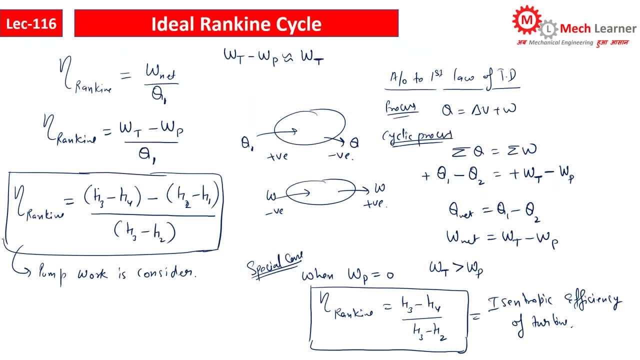 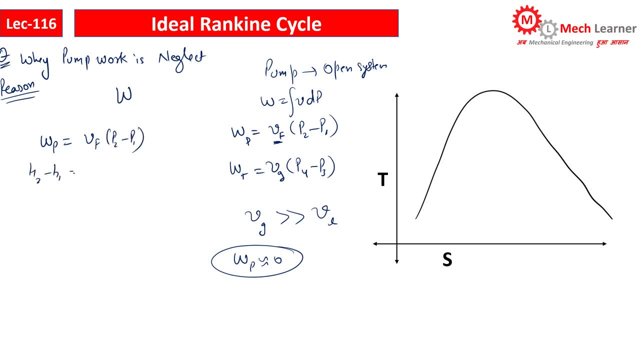 the expression we just derived. that is equal to H2 minus H1.. So P2 minus P1.. And this is H2 minus H1. is equal to Vf plus P2 minus P1.. H2 is equal to H1 plus specific volume, P2 minus P1. 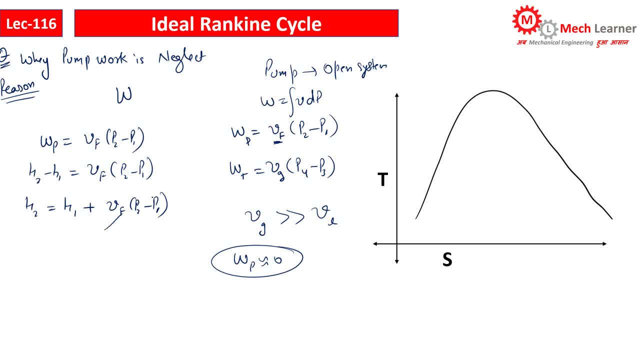 Specific volume is 0.00.. So if we assume 0, it will be cancelled out. If you write any value in it, when you multiply it with pressure, it will be approximately equal to 0. So H2 is equal to H1.. 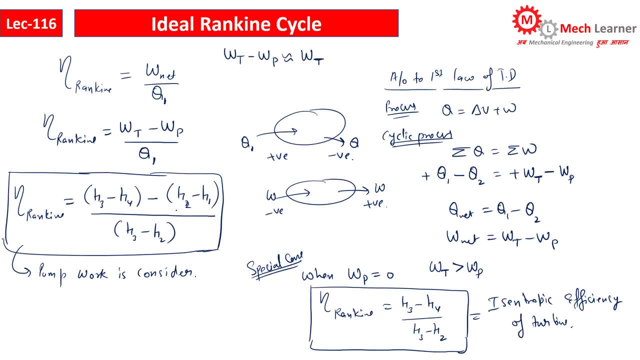 So here H2 and H1 are equal, So this term is cancelled out. So this is the efficiency of Rankine cycle when we neglect the pump work. So here the Rankine cycle is done. Let's see the TS diagram of the Rankine cycle. 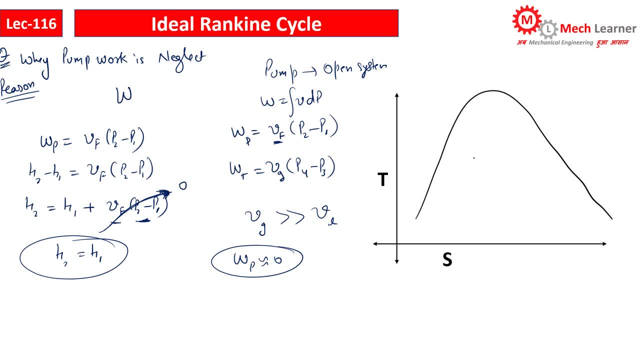 In this TS diagram, this curve is liquid plus vapor mixture And this is vapor And this is liquid. This is critical point. This is critical point. On this side of critical point, this curve is saturated vapor And on this side of critical point, 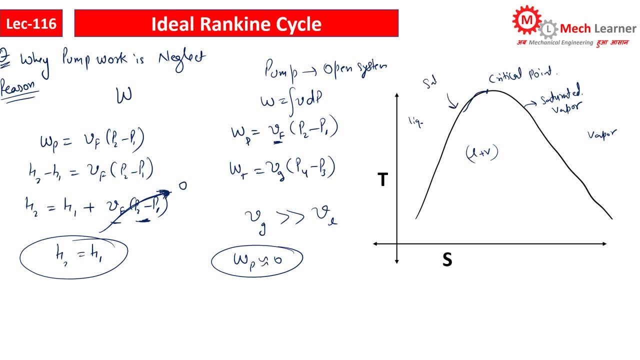 this curve is saturated liquid. Now let's make the TS diagram of the Rankine cycle. So first of all, see 1 to 2.. How is the pump? It is an isentropic compression process. Isentropic compression means: 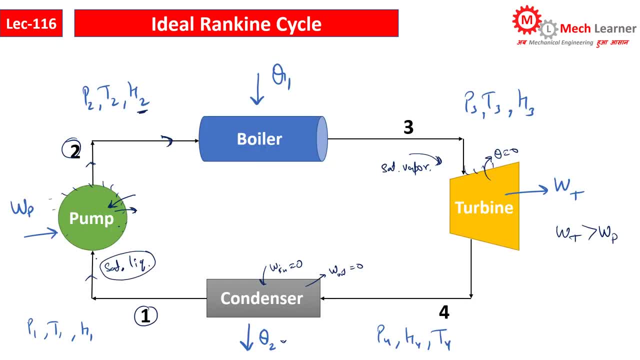 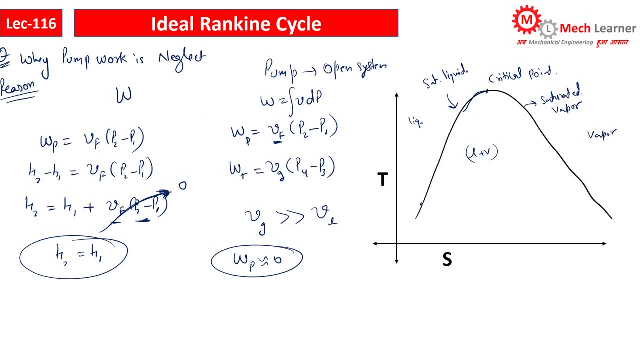 it will be an entropy constant And the working fluid in it is saturated liquid. This is saturated liquid, So saturated liquid will start from here. It is an entropy constant, So entropy constant will be a straight line. This is a straight line. 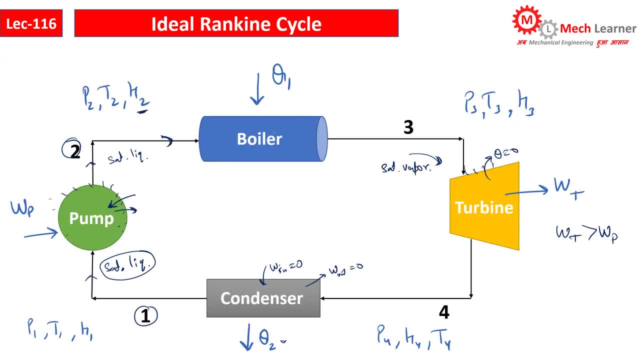 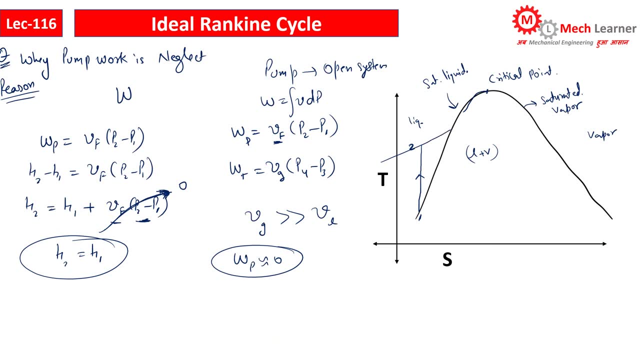 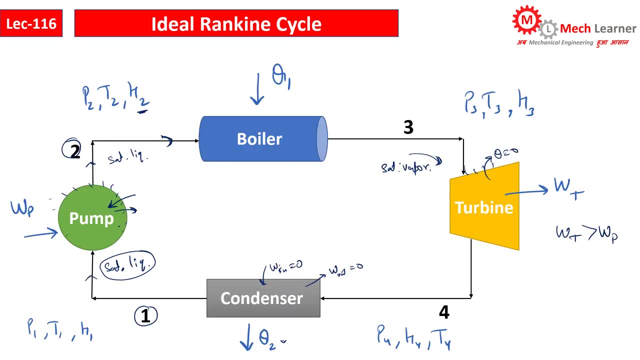 This is 1 and this is 2.. In boiler we add heat on constant pressure. So constant pressure is made in this way. in TS diagram This is the line of constant pressure. So this is second And this is the third point. 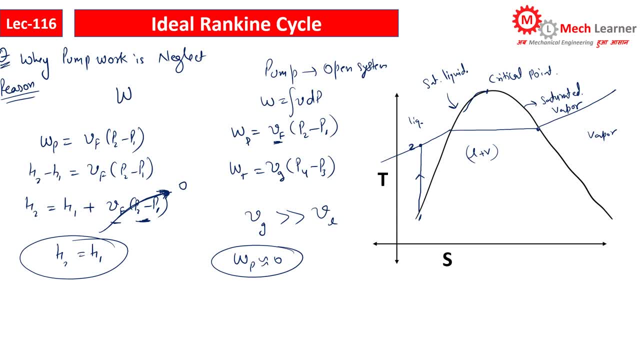 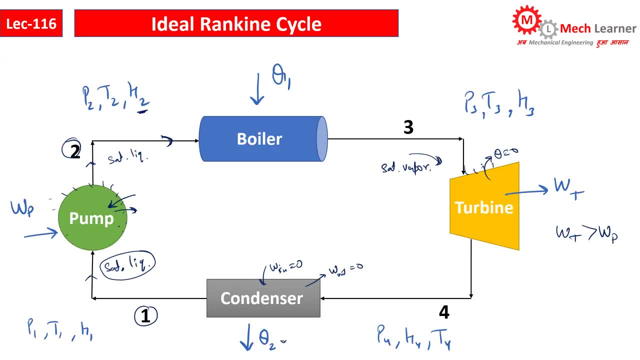 And this is saturated vapor. So saturated vapor will be this point. So second is 2.. And this is the third point. Saturated vapor is now 3 to 4.. Isentropic expansion process. Isentropic means entropy constant. 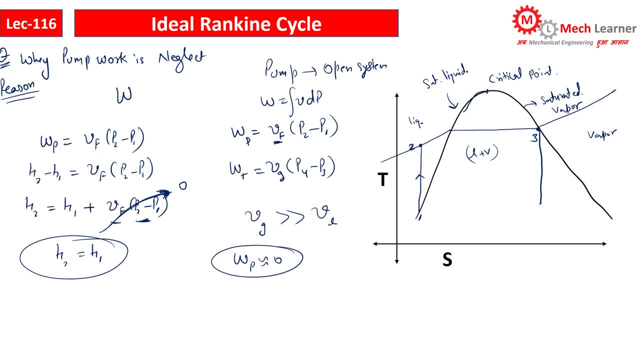 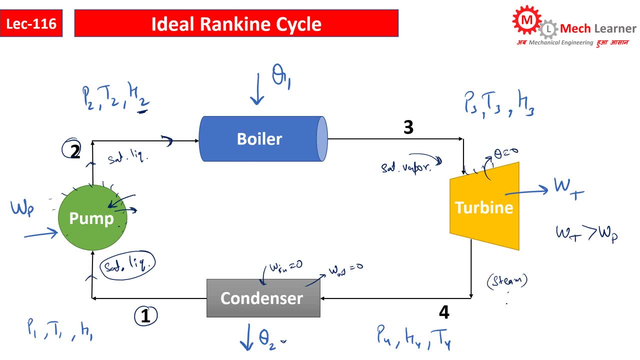 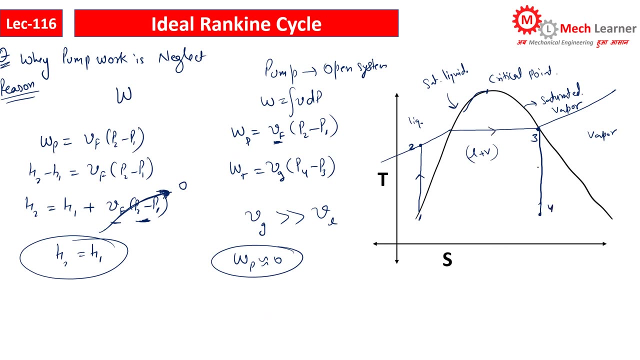 Entropy constant. When vapor comes out of the turbine, we call it steam. Now, in steam there is also liquid and vapor. This steam is of liquid plus vapor mixture. So this is our fourth point: Isentropic expansion. 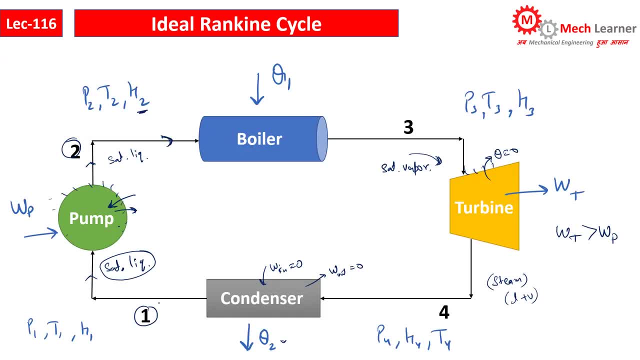 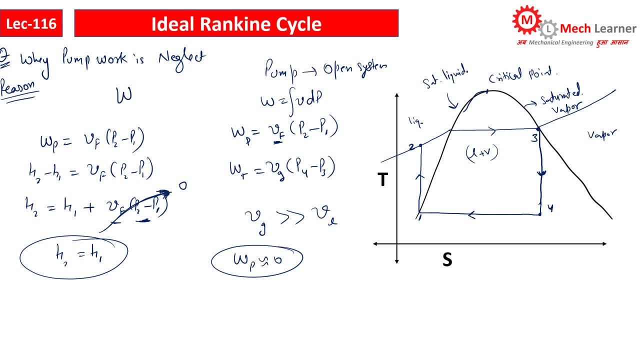 After that, condenser In condenser, we reject heat. So what will come again? Steam will come on saturated liquid. Okay, Like this. Okay, So in 3 to 4, WT, In 1 to 4, heat is being rejected. 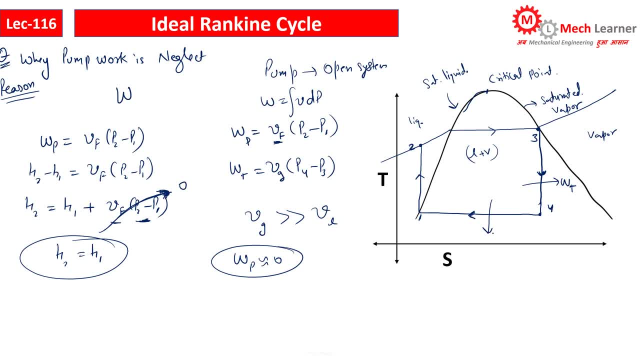 This is QT, This is Q2.. Okay, And in 2 to 3, heat is being supplied. So this is Q1.. And in 1 to 2, we are supplying work, So this is WP, Okay. 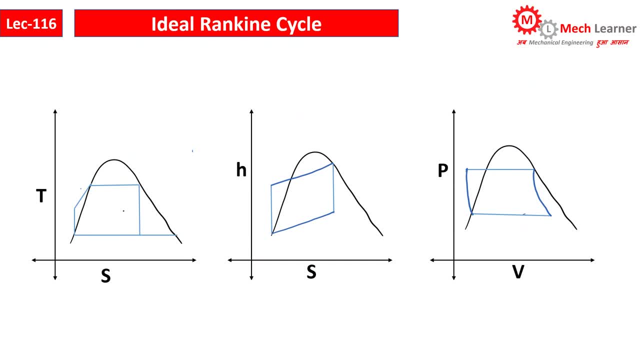 So this is TS diagram, This is HS diagram And this is PV diagram. Okay, This is 1,, 2,, 3,, 4.. So these are the 4 ideal rankine cycles: TS diagram, HS diagram and PV diagram. 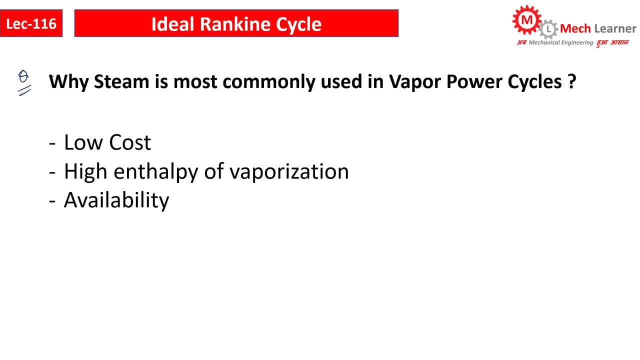 Okay, Next we will discuss this question. Why is steam most commonly used in vapor power cycle? Why do we use steam? Because it is low cost, It has high enthalpy of vaporization And it is easily available. Okay. 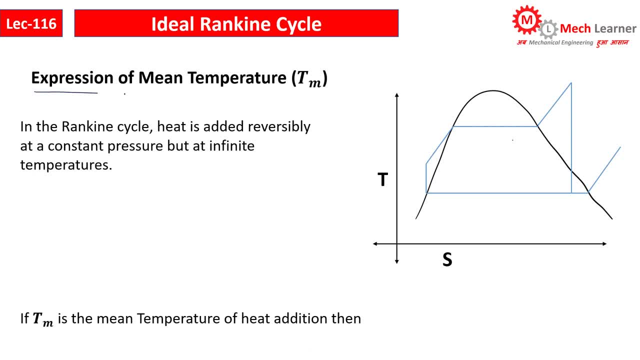 So we use steam in vapor power plant. Next we will calculate the expression of mean temperature. Mean temperature is denoted by Tm. We are calculating mean temperature because the efficiency of rankine cycle depends on mean temperature. If we increase mean temperature, efficiency of rankine cycle will also increase. 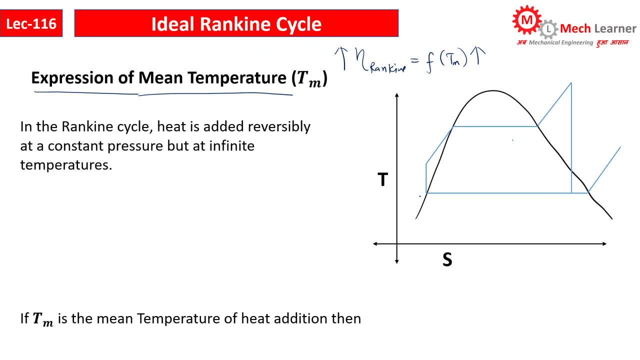 Okay, This is TS diagram of rankine cycle. This is 1., This is 2., This is 3. And this is 4.. Okay, Now we will understand what is mean temperature. In rankine cycle, heat is added reversely. 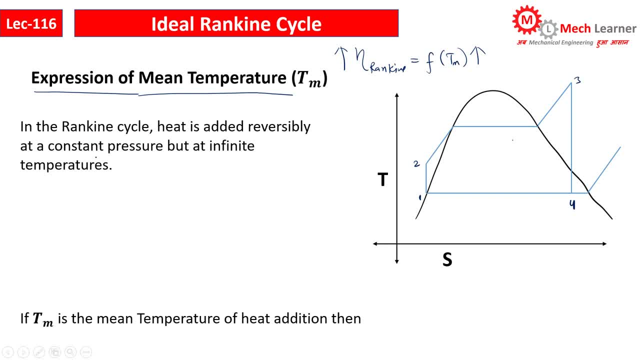 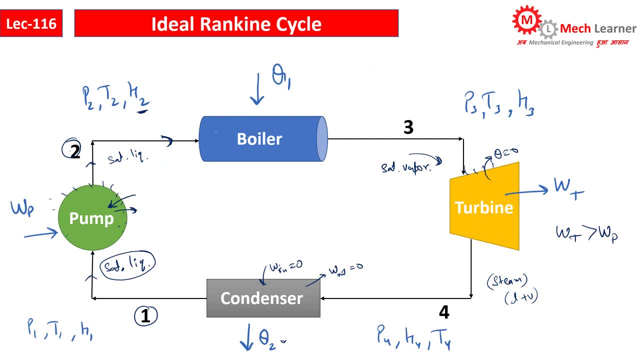 Heat is added reversibly at a constant pressure, But at infinite temperature. What does this mean? We are supplying heat in boiler, We are supplying heat of Q1 amount. And what is this process? 2 to 3.. 2 to 3 means isobaric heat addition process. 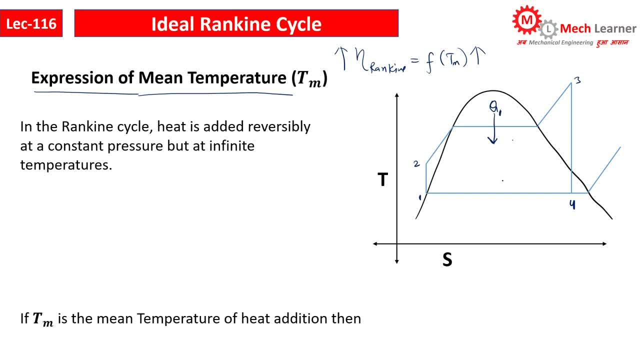 Okay, 2 to 3. isobaric heat addition process: Q1: amount of heat is added in this Heat is rejected in 1 to 4.. Okay, So here temperature is varying in 2 to 3.. First it changed from here. 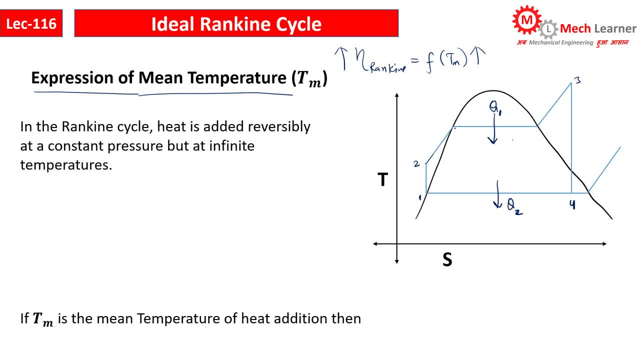 Then it is constant. Then it is like this: Okay, It is changing like this, Then it is constant, Then it is changing like this: Okay, So this is called infinite temperature. Okay, So in this way, we take one temperature like this: 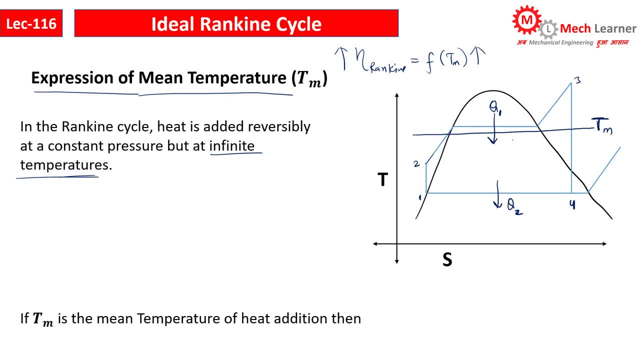 This is mean temperature. Okay, So in rankine cycle we consider mean temperature like this. Meaning efficiency of rankine cycle is equal to 1 minus. See what is the efficiency of Carnot cycle. The efficiency of Carnot cycle is 1 minus. 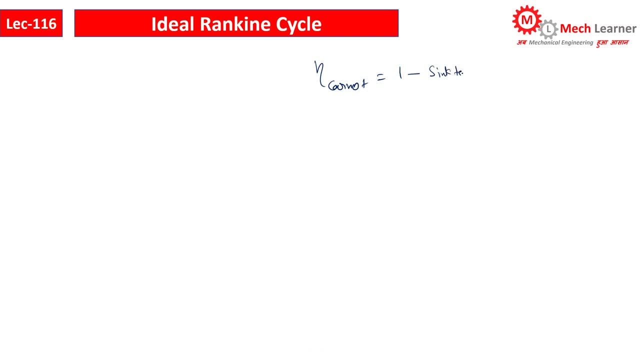 This is sink temperature, Okay, And this is source temperature. Okay. This is 1 minus T3 is the sink temperature. The source temperature is T3.. Source temperature is T3.. Okay, It is sink temperature At a height where the heat is getting rejected. this is 4.. 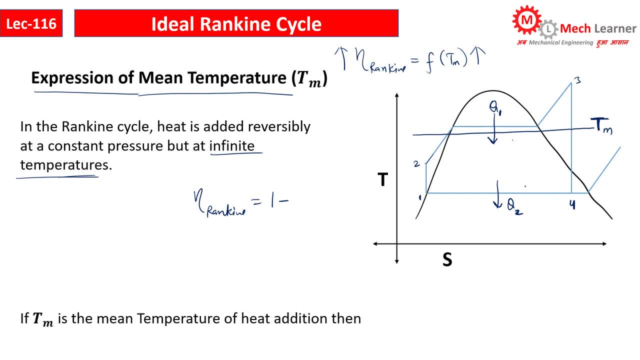 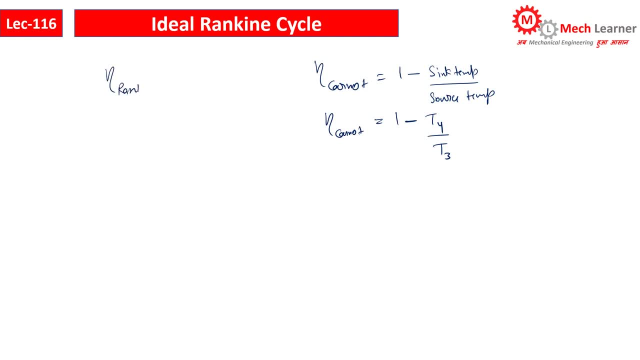 Okay, So this is T. This is the efficiency of Carnot cycle, See. look at the efficiency of rankine cycle. The efficiency of Rankine cycle is equal to 1 minus Sink temperature is the same as T4. Okay. 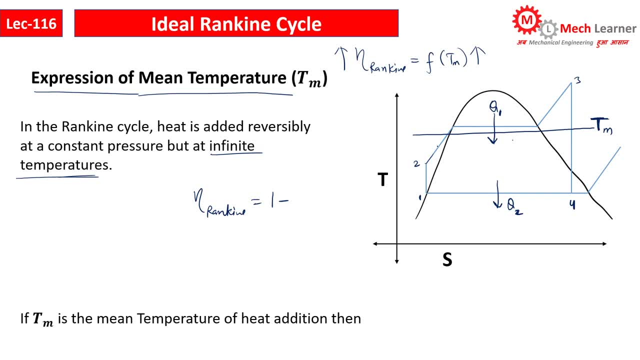 But the source temperature here is like this: See, the source temperature here is changing in this way, Then it is getting constant, how it is changing. then it is getting constant, then it is changing. so what we do is we consider the mean temperature. 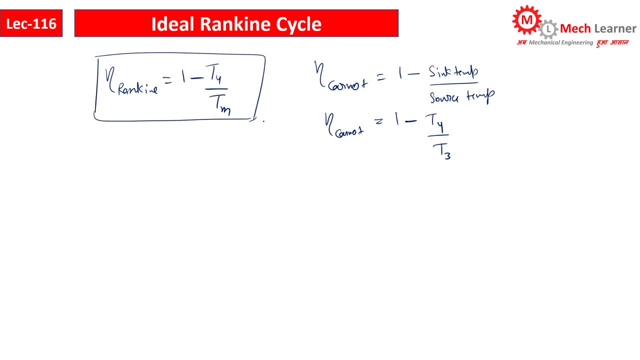 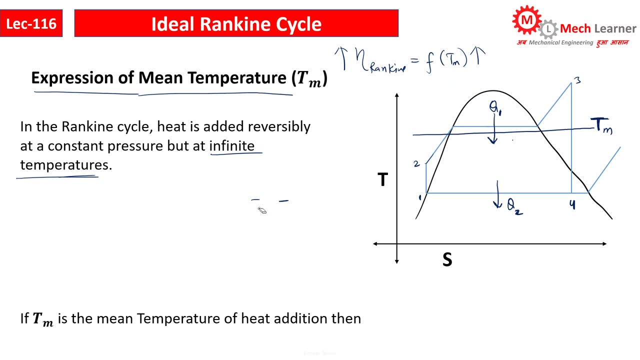 so this is the efficiency of its Rankine cycle and this is the efficiency of its Carnot cycle. now see how we will get the expression of mean temperature. let's remove this: the amount of heat supply in the boiler. its expression is H3-H2, which we just tried. 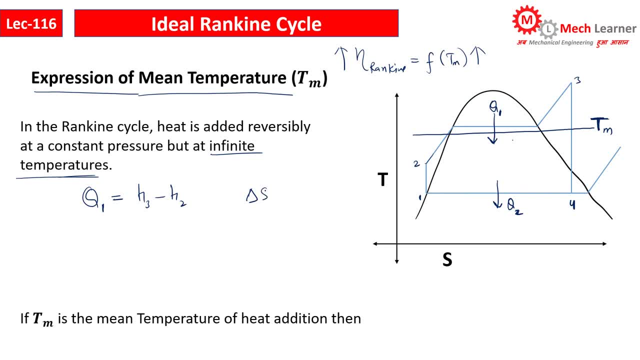 now see here the entropy delta S is equal to Q1 divided by. here the temperature is varying in 2-3 processes. so let's take the mean temperature now. delta S in 2-3 processes S3 is equal to S4 because it is an isentropic process. 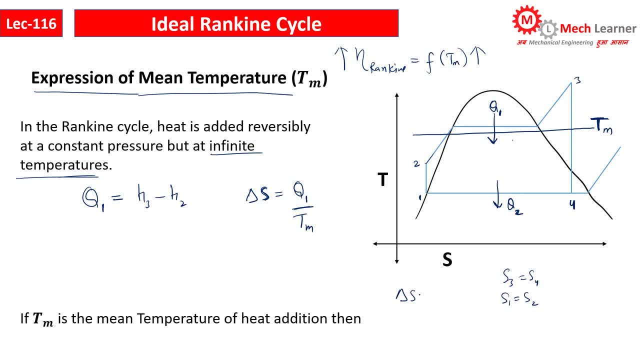 entropy will be constant on 1 and 2, so we can write delta S as S4-S1. this is delta S. change in entropy: this is S4-S1, and Q1 value is H3-H2. this is Tm, so mean temperature is equal to. 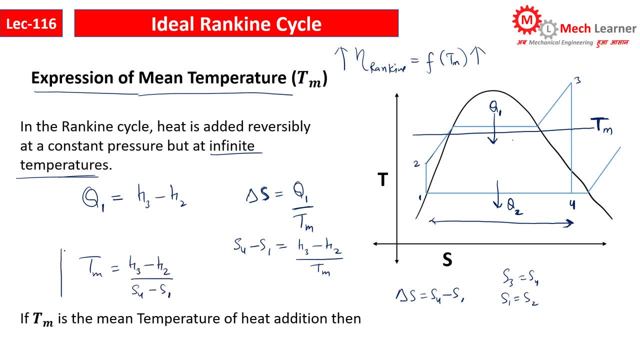 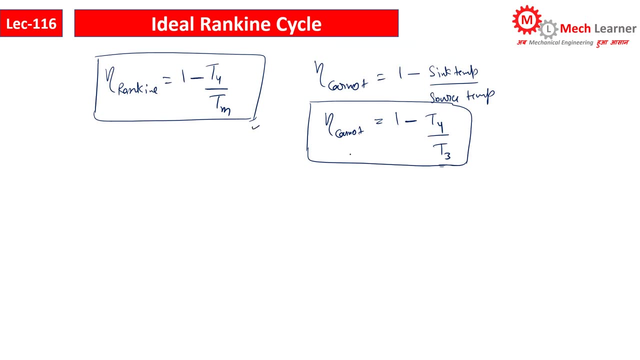 H3-H2, this is S4-S1. this is the mean temperature. at this temperature we add heat. at this temperature we add heat in the Rankine cycle. so this is the mean temperature. now see the efficiency if we compare the efficiency of the Rankine cycle. 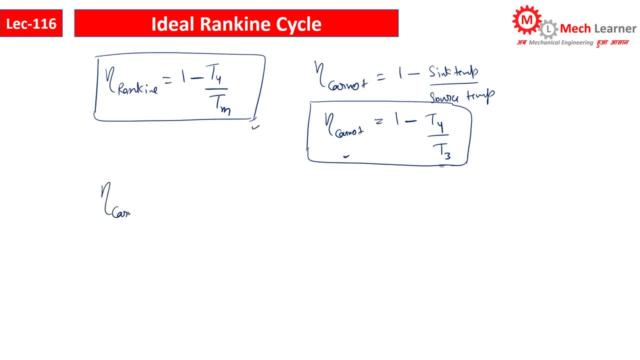 or the Carnot cycle, whose efficiency will be greater. Carnot cycle's efficiency is maximum as compared to Rankine and let's see the reason. if we compare in T3 and Tm, T3 is this and this is Tm, so T3 is greater than Tm. 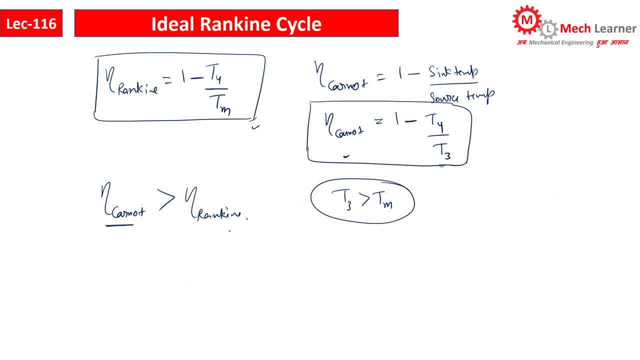 so when you add value, Carnot cycle's efficiency will be maximum and Rankine cycle's efficiency will be lower. so efficiency of Rankine cycle is lower than efficiency of efficiency of Carnot cycle. so if we want to increase the efficiency of Rankine cycle, 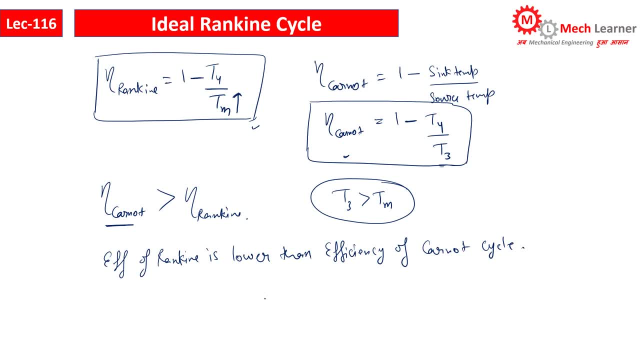 then we have to increase the mean temperature. so efficiency of Rankine cycle is the function of mean temperature, is the function of mean temperature. note it down: higher the mean temperature, higher the mean temperature, higher will be the efficiency. so remember the efficiency of Rankine cycle increases at mean temperature. 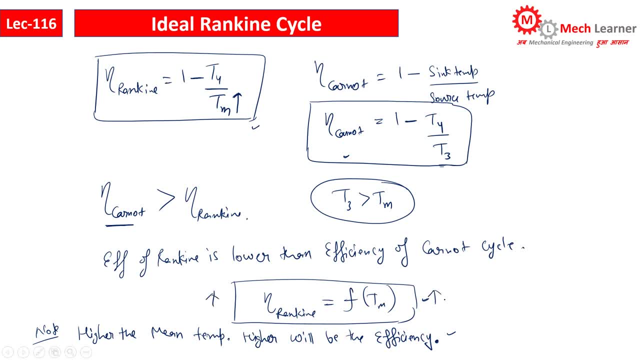 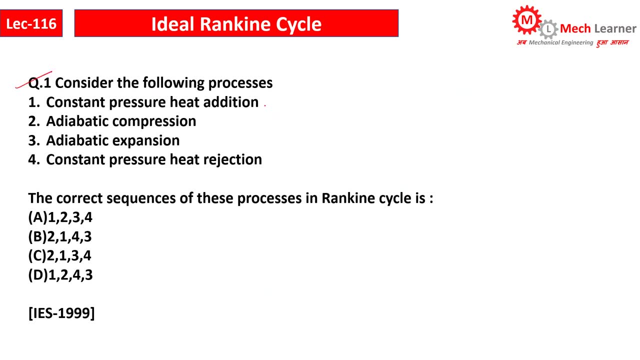 if we want to increase the efficiency, then we have to increase the mean temperature as well. next we will discuss numerically question no.1. consider the following process: total 4 processes: are there constant pressure, heat addition, adiabatic compression, adiabatic expansion. 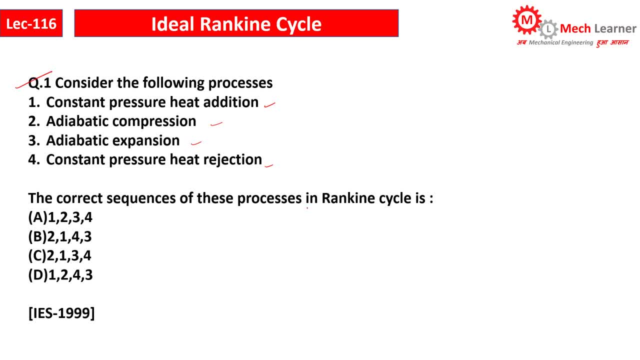 constant pressure, heat rejection, the correct sequence of these processes in Rankine cycle. in Rankine cycle we have to tell the correct sequence. so in Rankine cycle, boiler, boiler working fluid goes to turbine, turbine to condenser, condenser to pump. this is cycle. 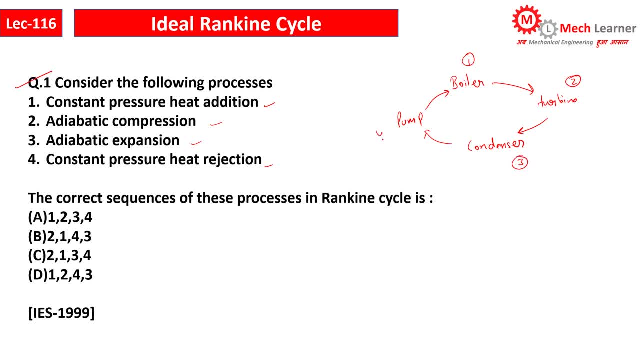 so this is 1,, 2,, 3, and 4. boiler boiler: constant pressure heat addition boiler is constant pressure heat addition. constant pressure heat addition process turbine has adiabatic expansion. adiabatic expansion. this is 3rd. 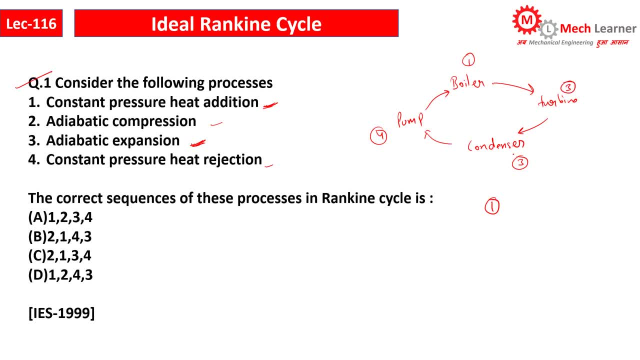 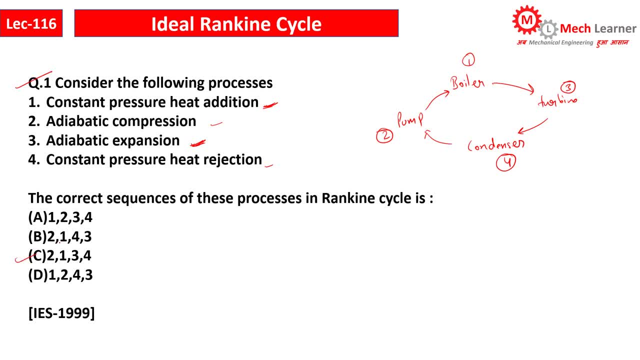 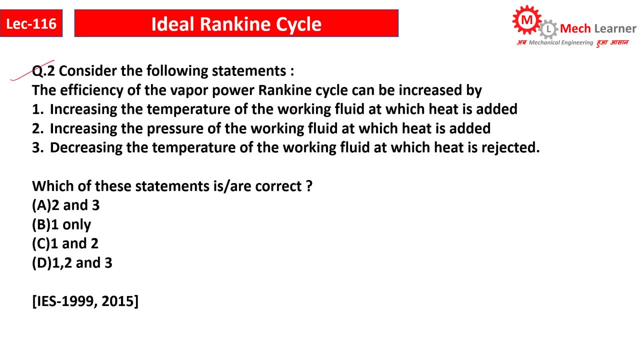 2,, 1,, 3,, 4, then 2, so C option is correct. let's see the next question, question no 2. consider the following statement: the efficiency of the vapor power Rankine cycle can be increased by increasing the temperature of the working fluid at which heat is added. 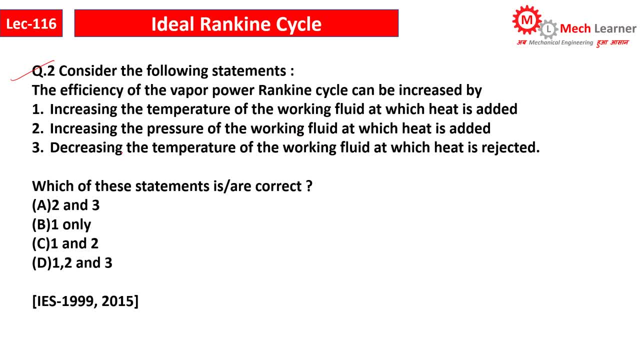 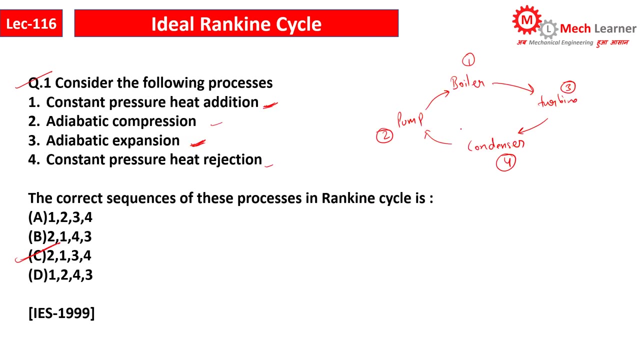 increasing the pressure of the working fluid at which heat is added, decreasing the temperature of the working fluid at which heat is added or reducing the pressure of the working fluid at which heat is present. so when there is an animated, F1, F2, F3, F4. 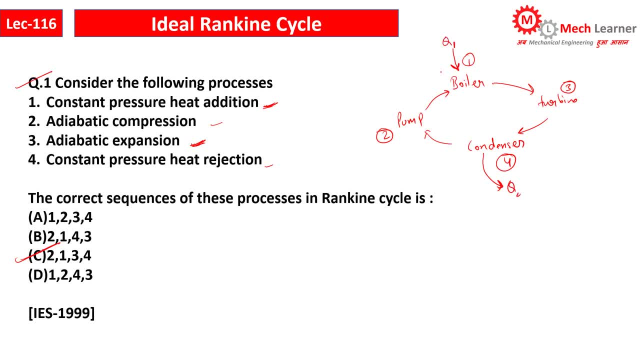 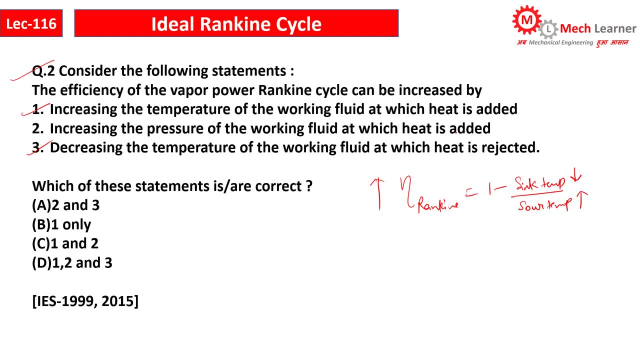 F5, F6, F7, So these two options are absolutely correct. Let's read the second part: Increasing the pressure of the working fluid at which heat is added. The temperature at which we are adding heat, the pressure should also increase there. 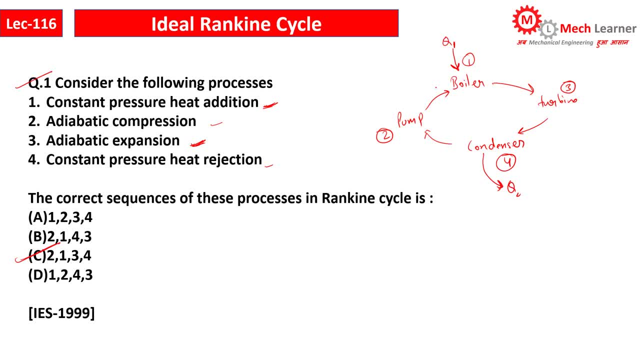 That is why we have put a pump here, Because it is converting low pressure into high pressure. So high pressure, high temperature. when the steam comes in contact with the turbine, then our electricity is generated. So if we want to increase the efficiency, 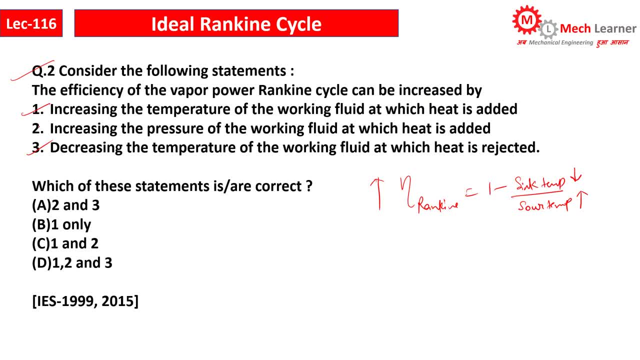 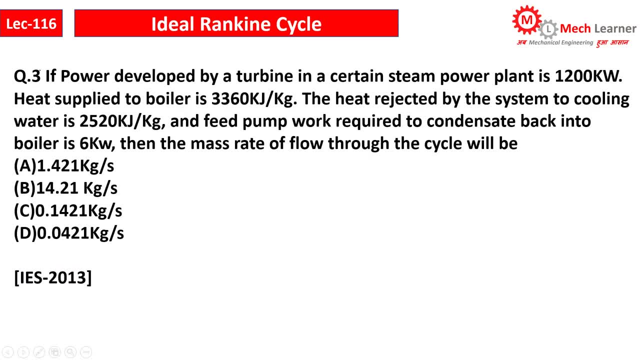 then we will have to increase the temperature and pressure in both In the boiler. So the second is also correct. Its D option is correct. Let's see the next question, Question number third: If power developed by a turbine in a certain steam power plant, 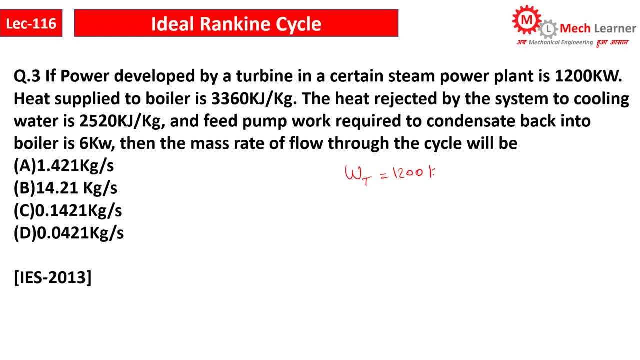 the turbine work is given 1200 kilowatts- Okay, It is generating this much. Heat. supply to boiler is 3360 kilojoules per kg. Heat ejected is 2520 kilojoules per kg. Feed pump work required to condensate back into the boiler is 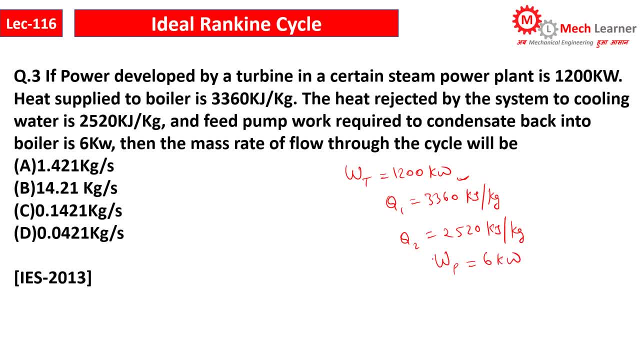 3360 kilojoules per kg. Pump work is 6 kilowatts. Okay, Then the mass rate of flow through the cycle will be: We have to calculate the mass flow rate. Okay, We have to calculate the steam flow rate in the entire Rankine cycle. 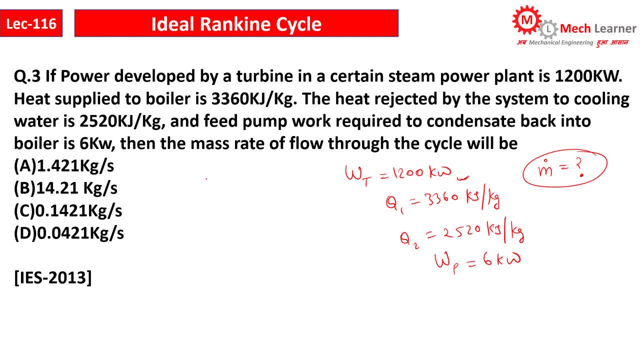 Okay, So look at the expression in this. If we apply the first law of thermodynamics to the entire Rankine cycle, then it will be like this: Net work done is equal to net heat supply. Okay, Work done is turbine work minus pump work. 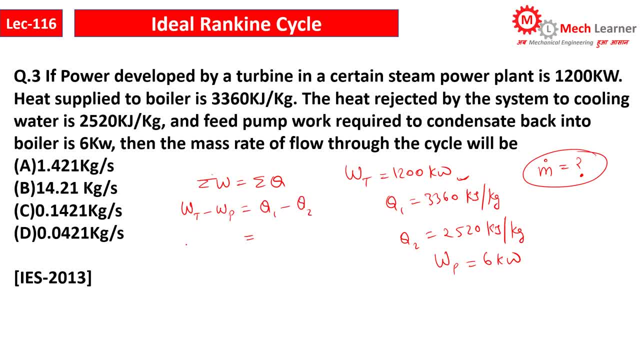 And that is equal to Q1 minus Q2.. Okay, What is the turbine work? It is 1200 minus 3360.. Q1. Now look here. It is kilojoules per kg. So if we multiply it with the mass flow rate, 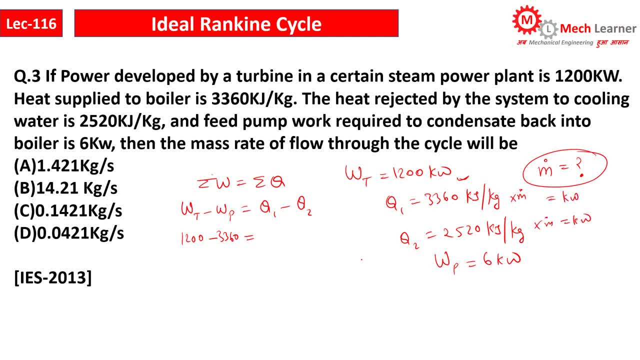 then it will be in kilowatts. Okay, So m dot and this is 3360 minus 2520.. Okay, So from here the mass flow rate will be 1.421 kilojoules per second. Okay. 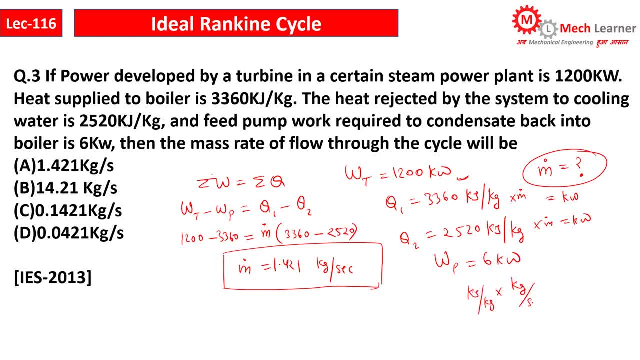 Look here It is kilojoules per kg. So from here we will get Kg per second. So Kg to Kg is cancelled out. Kilojoules per second. Kilojoules divided by second, This is 1 kilowatt. 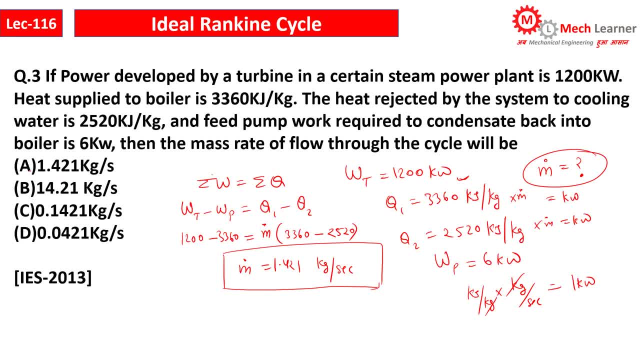 Okay, That is why we multiplied it with the mass flow rate. Okay, So the third A option of it is correct. Let's see the next question, Question number 4.. An electric power plant produces 10 megawatt of power. 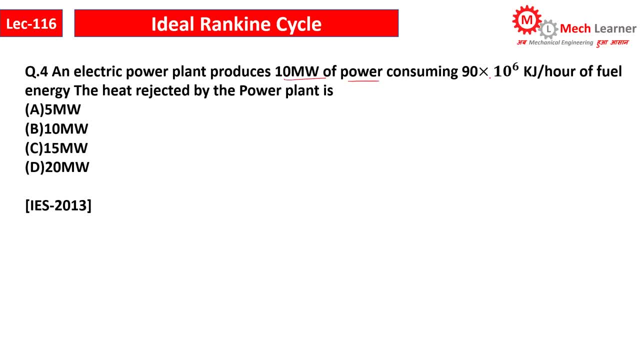 consuming 90 to 10 to the power of 6 kilojoules per hour of fuel energy. Fuel energy means the amount of heat that we have supplied: 90 to 10 to the power of 6 kilojoules per hour. 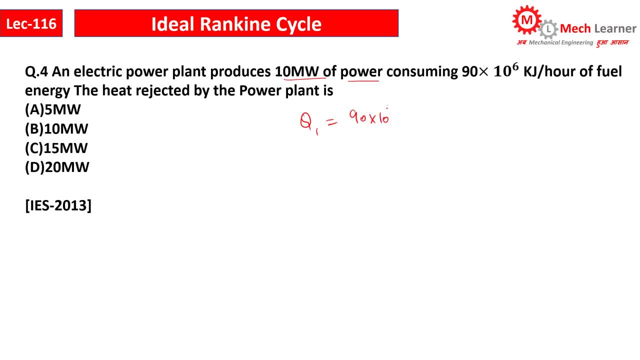 Okay, And 90 to 10 to the power of 6 kilojoules per hour. Okay, And 90 to 10 to the power of 6 kilojoules per hour. Okay, And net work done. How much power are we getting? 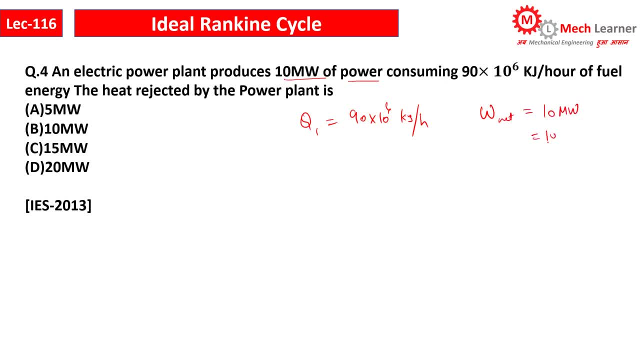 10 megawatt. We will convert it into kilowatts, So this is 10,000 kilowatts. How much heat is ejected? We have to get that Net work done. So see here Power. Who will get the power? 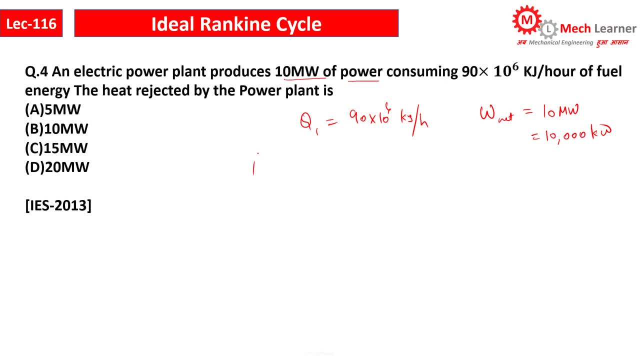 Q1 minus Q2 will get the power. Okay, What do we have to get? We have to get Q2.. This is Q1 minus power. Okay, Q1 is 90 to 10 to the power of 6 kilojoules per hour. 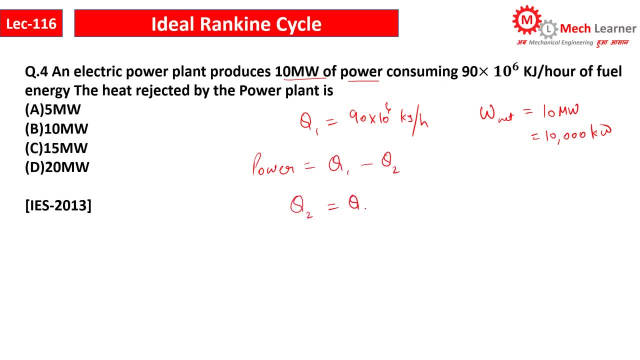 We have to change it to seconds. Okay, We have to get Q2.. This is Q1 minus power. Okay, Q1 is 90 to 10 to the power of 6 kilojoules per hour. We have to change it to seconds. 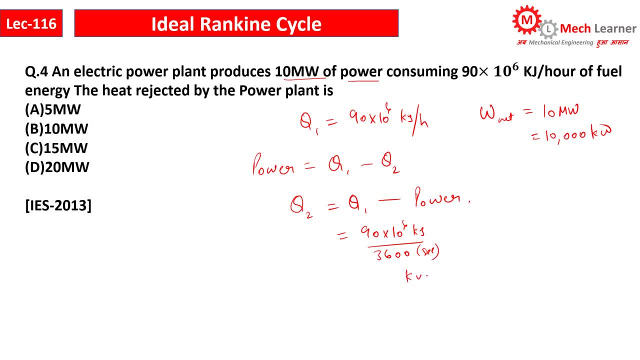 This is how units are Okay. Kilojoules per seconds. It will be kilowatt. You had just told Minus. How much power is there? Okay, Net work done. This is equal to power, Okay. 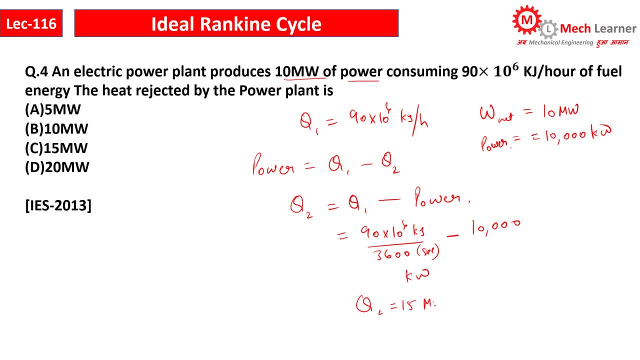 So we will solve it. So from here, 15 megawatt- 15 megawatt amount of heat- will get ejected. So 4th's C option is correct, Okay. So from here, 15 megawatt amount of heat will get ejected. So 4th's C option is correct. So 4th's C option is correct. So 4th's C option is correct.